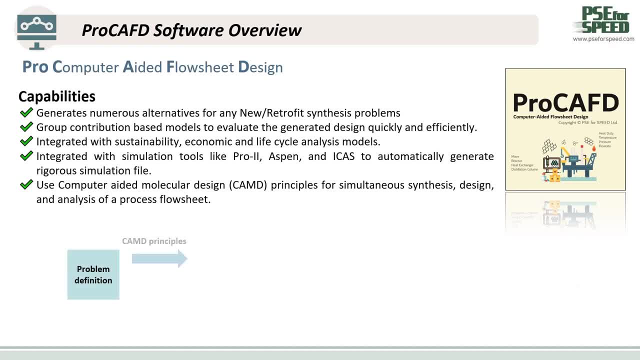 First, when the problem is defined by using the CAMD principle, the program will generate the functional group. but then it will combine the group together And then it will give the feasible molecule and then it will screen the molecule using the property model. 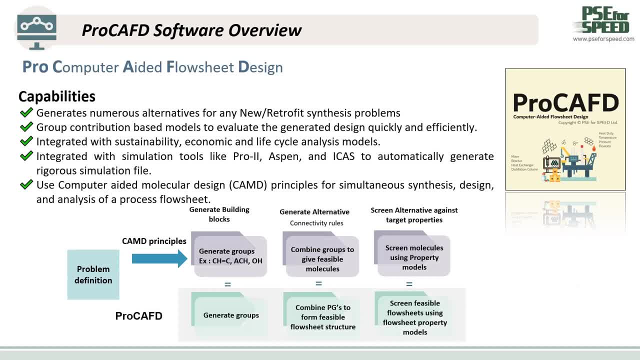 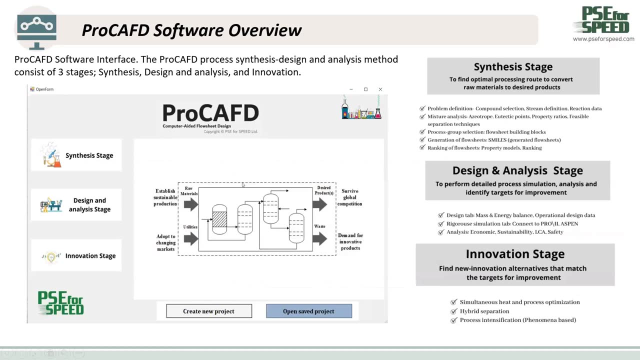 In the same way, the PRO-CAFD will generate the group and then it will combine the process group to form the feasible flow sheet structures And then the program will screen the feasible flow sheet using the flow sheet property model. This picture here shows the software interface of the PRO-CAFD. 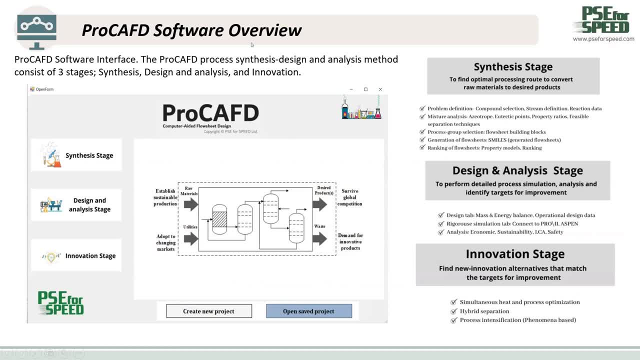 which you can see that the program has consists of two components. The program has consists of three stages: The synthesis stages, the design and analysis stages and the innovation stages, which the detail of each stage has already been explained in the professor's graphic lecture. 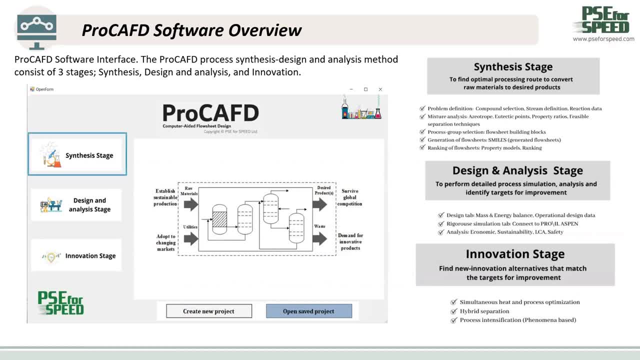 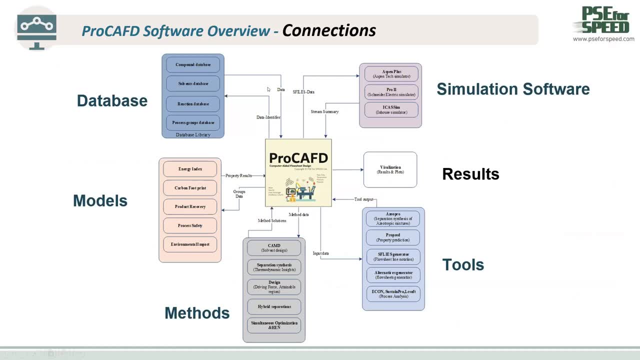 So in this presentation we're going to focus on the synthesis stages, But before that, this picture here shows the connection diagram of the PRO-CAFD, which tells the overview of how the program connects to the database, The lifecycle assessment, including the sustainability and the safety. 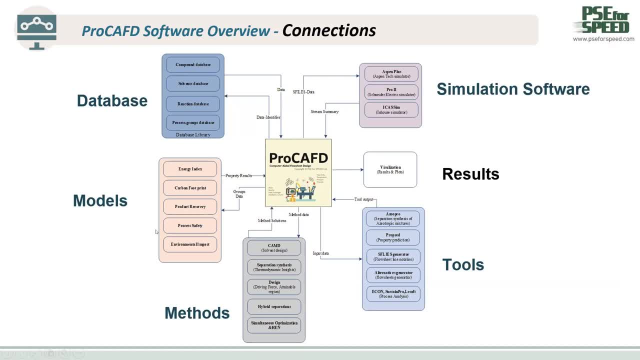 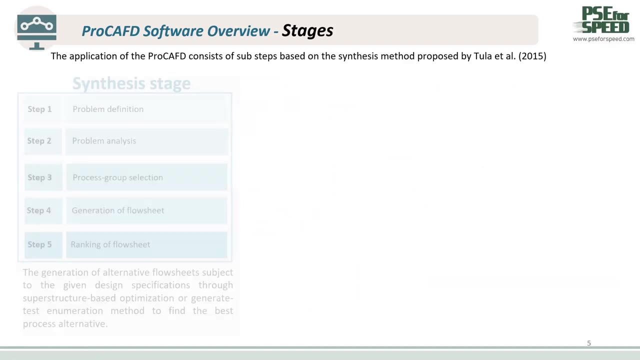 the simulation tool, the property estimation and also the process design. So that's why the PRO-CAFD is an efficient tool for the entire analysis. on the process design, As we mentioned earlier that the program has consists of the synthesis stages. 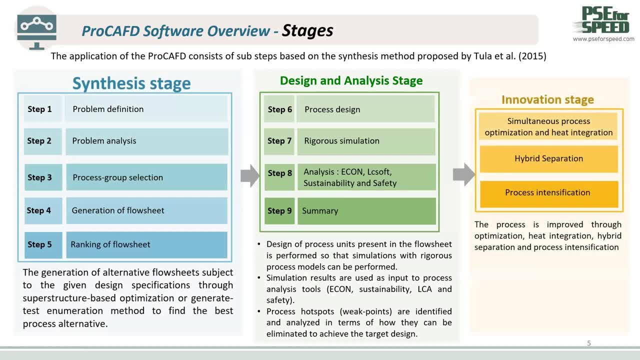 the design and analysis stages and the innovation stages, Then in this presentation we will mainly focus on the synthesis stages, and the design, analysis stages and innovation stages will be mentioned in the later session. So what is the task of the synthesis stages? 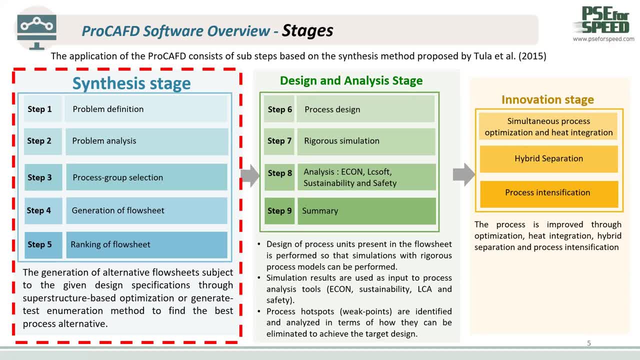 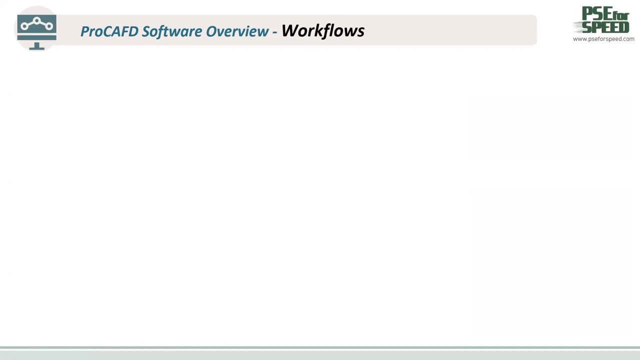 For the synthesis stages, the software will generate the alternative flow sheet, which is based on the design specification that the user has given in order to find the best process alternative. So now let me tell you the process. The process is the input, the target that the user needs to define. 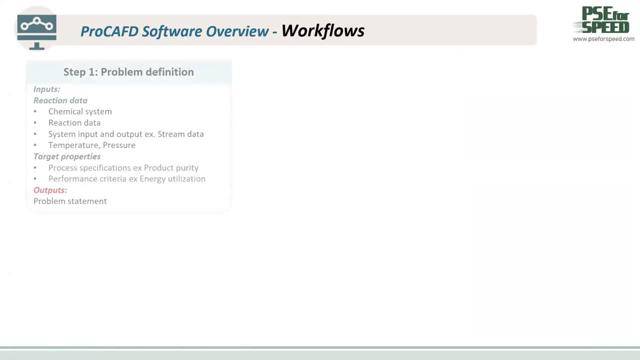 and the output that the program will generate in each step. First, the step one, the problem definition. the user needs to define the chemical system, the reaction data, the system input and output and the temperature And, moreover, the user needs to define the target properties, such as the process specification. 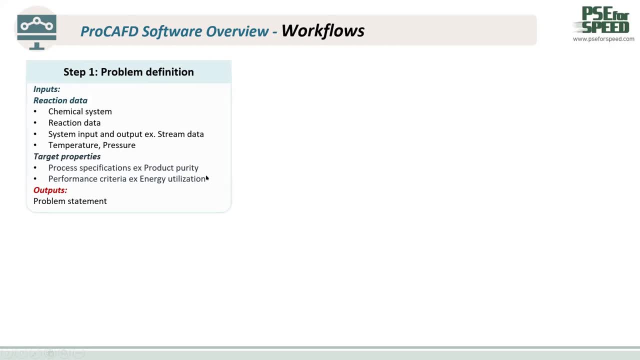 the process purity, the product purity and the energy utilization. So the problem statement will be created. Then for the step two, the problem analysis, the program. when the problem statement has been created, the program will generate the reaction analysis, the mixture analysis and the feasible separation, type identification. 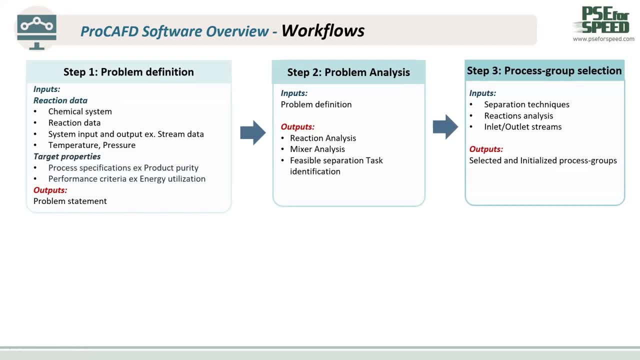 Then after that, for the step three, the program will take the information generated in the step two and it will create the initialized process group In the process. step four, the program will use the information of the initialized process group and generate the alternative flow sheet, which is stored in the form of the S-file. 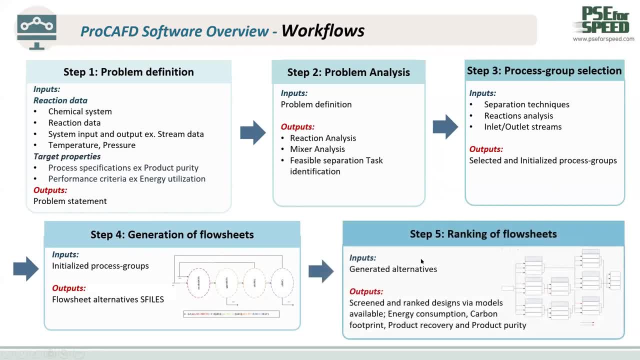 And after that, in step five, the program will screen and rank the alternative by using the available model. So in this step the user can rank the model in terms of the energy consumption, the carbon footprint, the product recovery and the product purity. 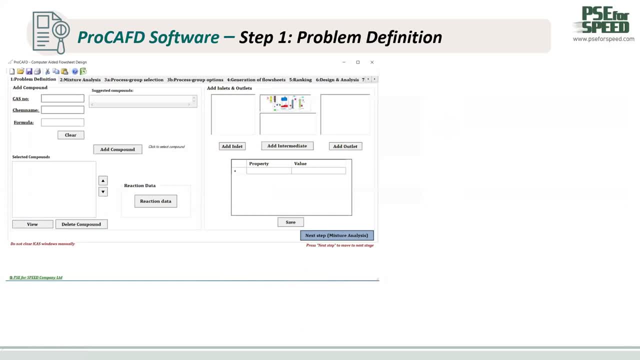 So now I want to show you how to perform the step one to step five. But before that, if you look at the picture carefully on the top of the bar, the user can know what step they are performing. But first let's start with step one. 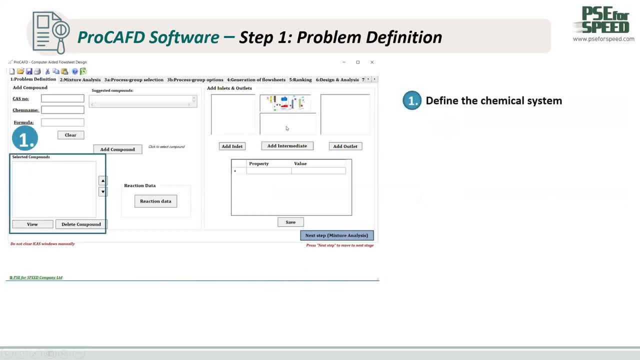 First, we need to define the chemical systems, such as the raw material and the product, And second, we need to give the reaction information. Then, after that, we need to define the steps. First, we need to define the system, input and output, such as the stream data. 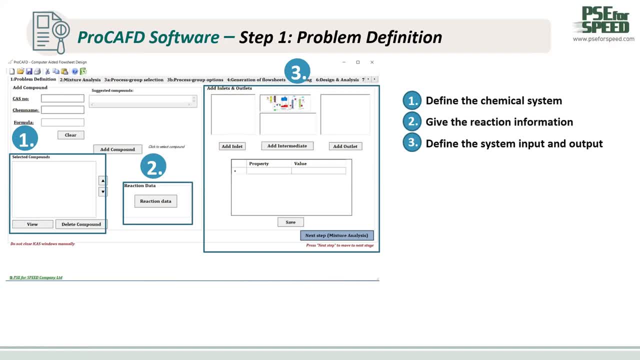 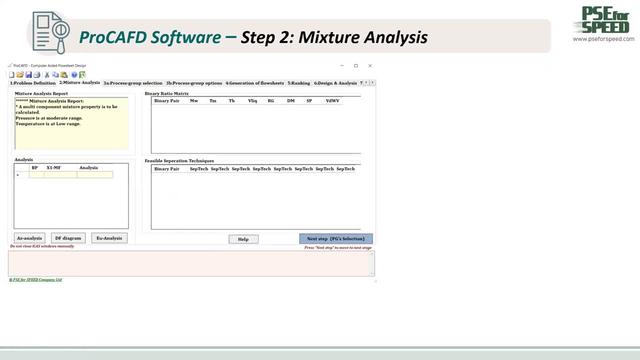 the stream composition, the pressure and the temperature. Then we click next, The program will create the problem statement And in this step the program will create the mixture analysis which first. the user can look at the mixture analysis report in this box. 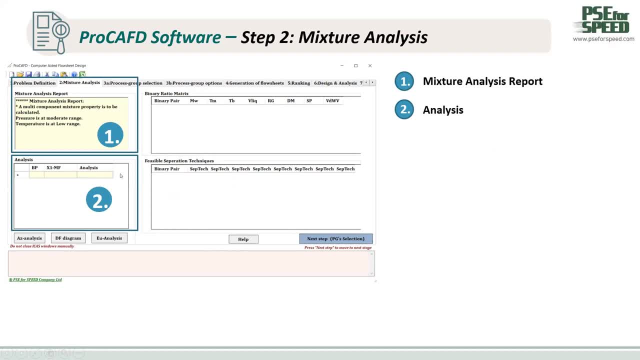 And then the second: the program will generate the analysis of the binary pair which the user can look at: the data of the azeotropic analysis, the drying pot diagram and the eudectic analysis. Then, third, the program will create the binary ratio metric. 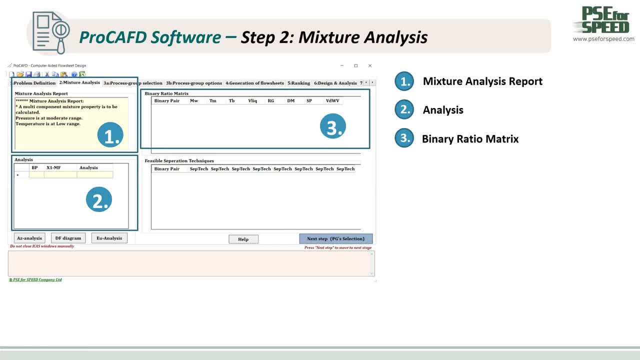 which the user can see the information of the binary ratio metric in the table. And fourth, the program will use the information from the binary ratio metric and the analysis of the binary pair to create the feasible separation technique. Then we click next And after that the program will use the information in the step two. 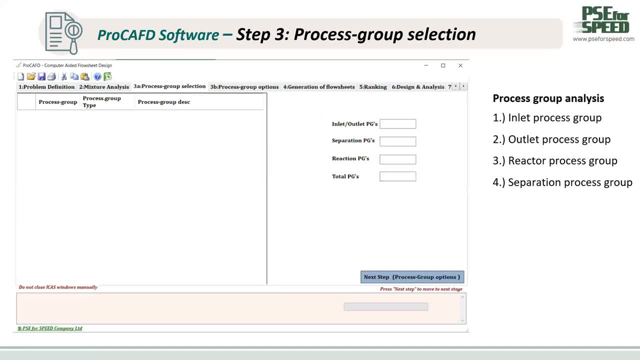 to create the process group, which consists of four process groups: the inlet process group, the outlet process group, the reactor process group and the separation process group, which will be presented in this box. In this step, the user can see the number of the process group. 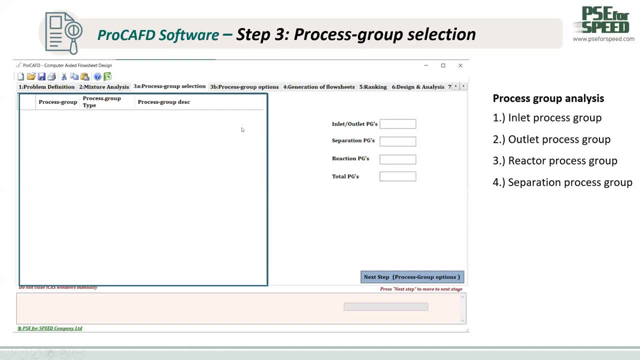 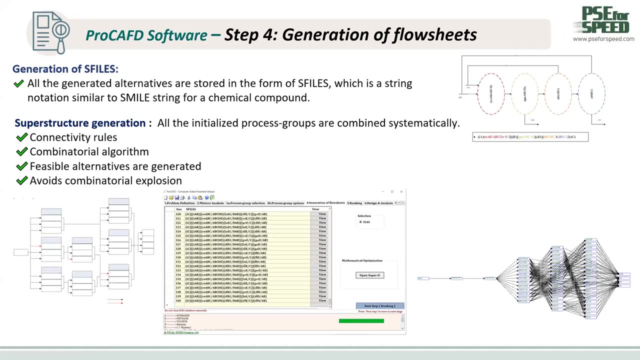 which we show in this bar. For example, if there are four inlet and outlet process groups, the program will show four in this bar. Then we click next. For the step four, the generation of flow sheet, the program will use the information from the process group. 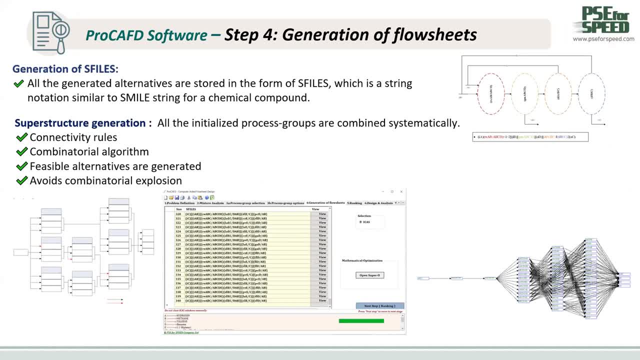 and create the flow sheet systematically based on the connectivity loop. just like the atom and molecule, The program will generate the possible flow sheet and store in the form of the S5, which. the S5 is the stink node, which is the rotation similar to the smile in string for the chemical compound. 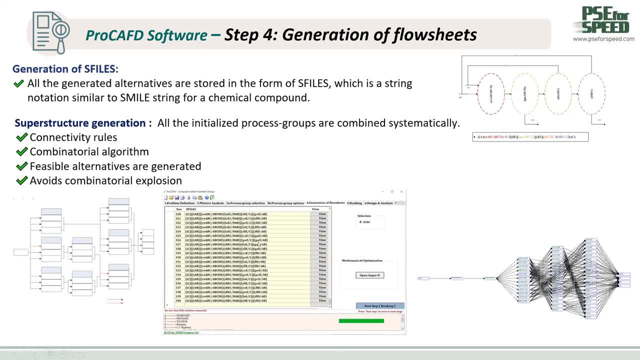 In this step, the program will list the alternative in this table and the user has the option that the user can click on open SuperO and the program will generate the superstructure of all the alternative. Moreover, the user can click on the View button. 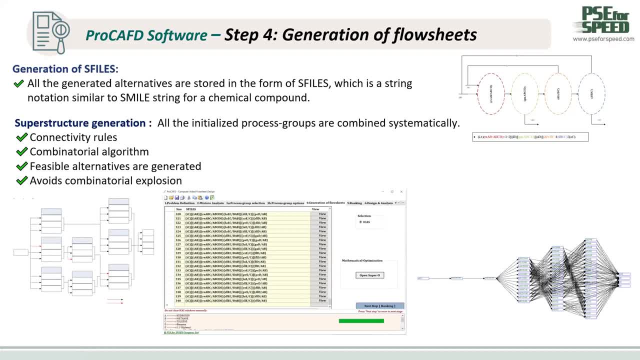 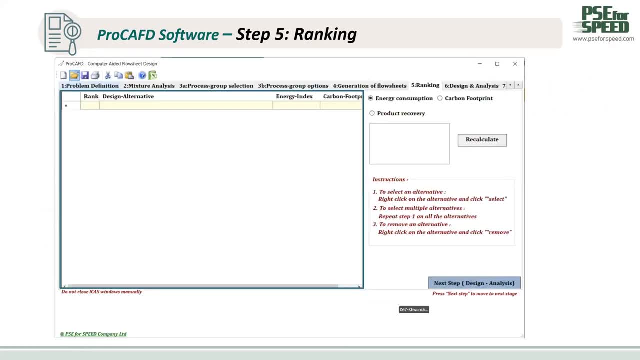 in order to observe the flow sheet of each alternative in ICAST program. Then we click next to step five. For the step five, the program will screen and rank the alternative by using the available model. In this step, the user can rank each model in terms of the energy consumption. 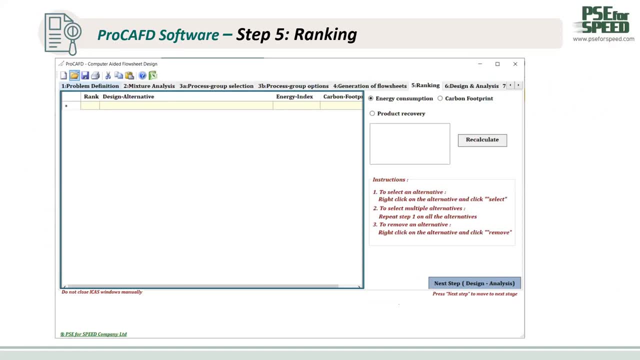 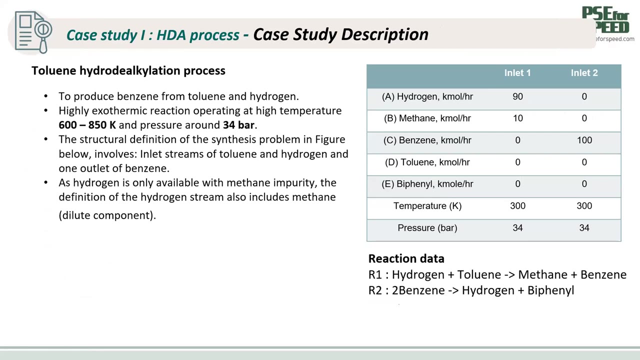 the carbon footprint, the product recovery and the product purity. So for the next step, I will show the example of the HDA flow sheet, which more detail of each step will be explained. The HDA process, or the toluene hydro-euclation process. 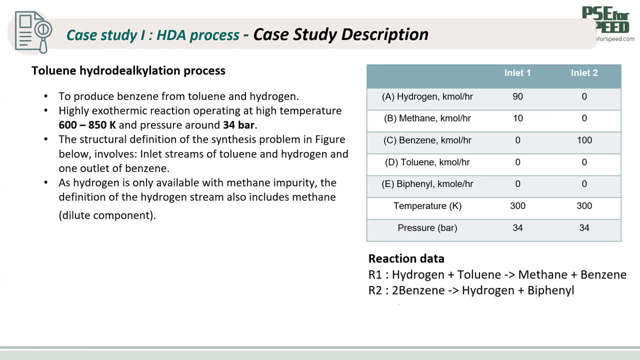 is the process that produces benzene from toluene and hydrogen, which. the reaction of this process is highly exothermic, which operates at approximately 600 to 580 Kelvin with the pressure of 34 bar. Since the HDA process has many alternatives that can produce benzene, 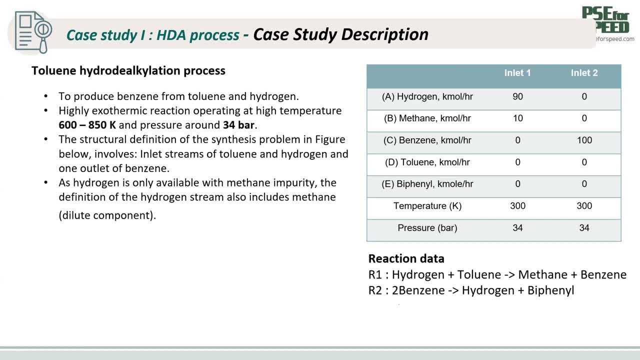 we can use the flow CFD in order to create more alternatives. First, we need to know the chemical system, which the chemical system is present in this table, such as the stream data, the pressure and the temperature, And second, we need to know the reaction data used in this step. 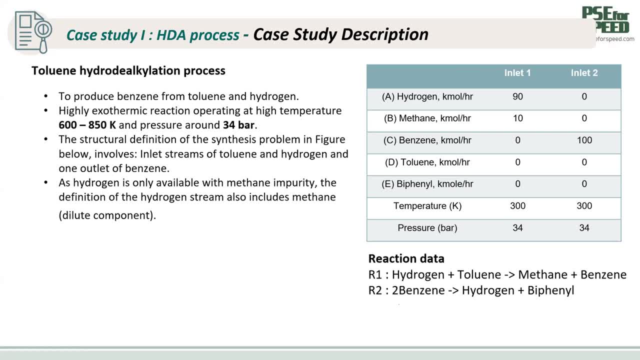 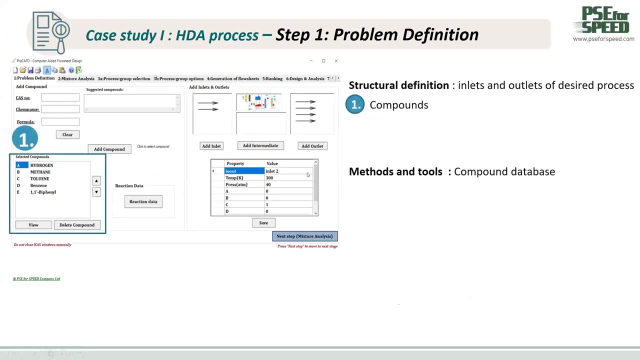 And all of this step will be demonstrated by Convano. First, for the step one, we need to define the chemical system, which is the compound used in the process. Second, we need to define the reaction data. And third, we need to define the system in the input and the output of the stream. 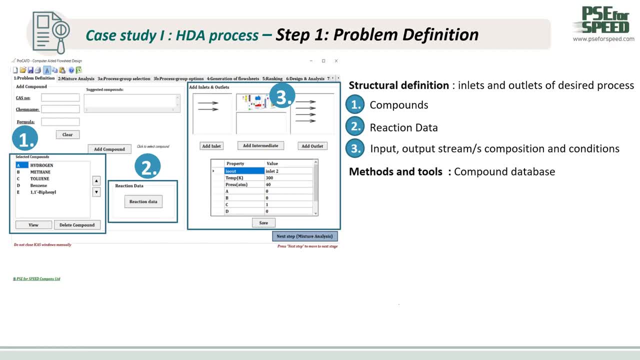 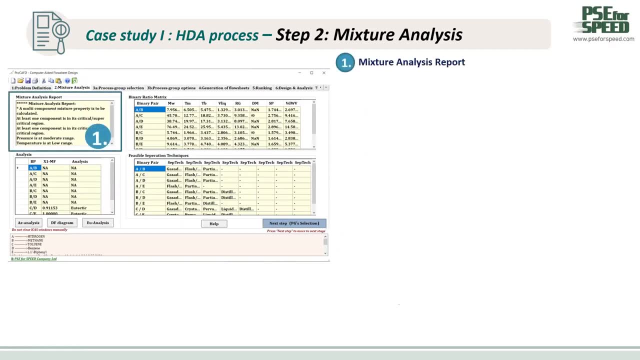 such as the stream data, the temperature and the pressure. Then the program will create the mixture analysis where the user can look at the mixture analysis report. The user can look at the analysis of the binary pair. The user can look at the information of the azeotropic analysis. 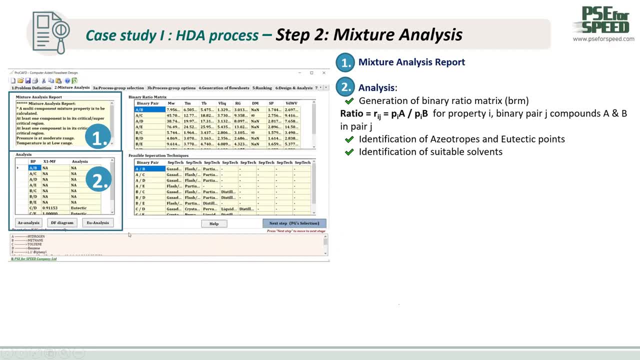 the drain force diagram and the unit analysis, And then the program will create the binary ratio matrix which in this process there are five compounds, so it means there are 10 binary pairs in total. In this table we show the property with respect to the binary pair. 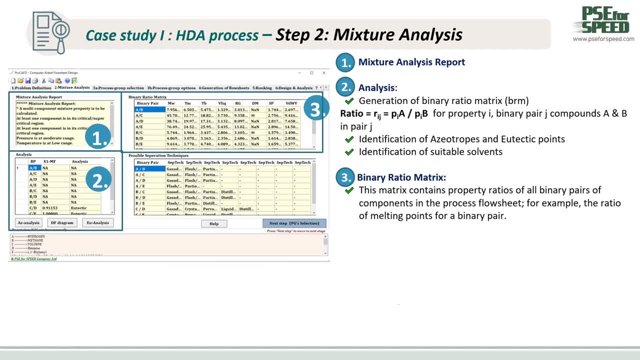 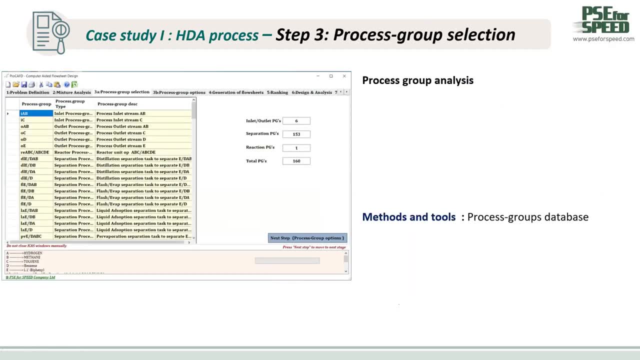 and based on the binary ratio matrix, the program can generate the feasible separation technique. Then we click next. The program will use the information from the previous step in order to generate the process group, which consists of the inlet process group, the outlet process group. 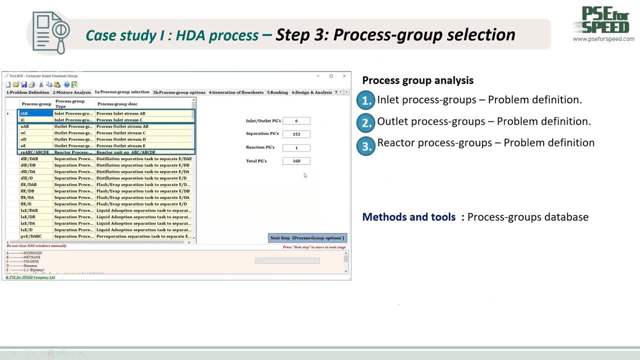 and the reactor process group. The information from this process group is from the step one And fourth, the separation process group with the data is from the step two. In this step the user can look at the number of the process group which is shown on the right bar here. 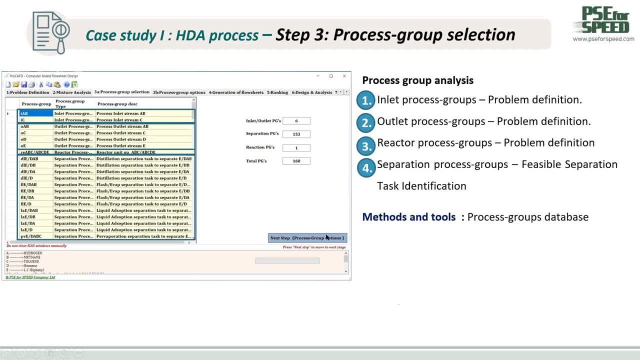 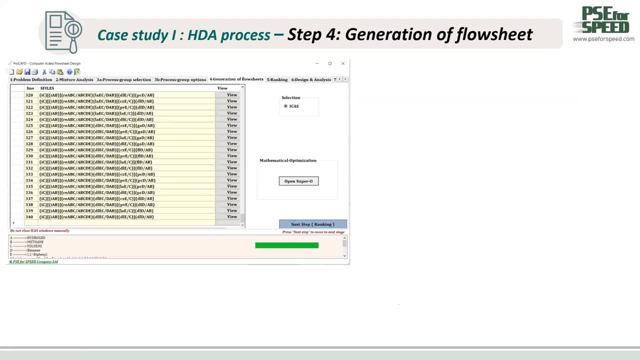 Then after that we click next, The program will use the information of the process group and generate the flow sheet systematically. like the add-on and normalization, The flow sheet system is the same as the SMILE program, which is stored in form of the S5,. 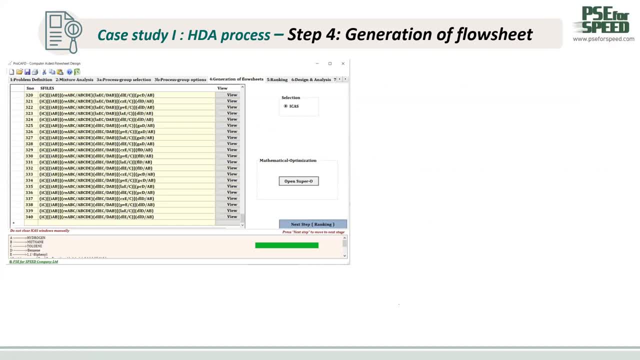 which the S5 is the nomenclature for the flow sheet, in the same way as the SMILE for molecular. The list of the alternatives will be presented here, which the user can click on: open super-all and the superstructure of all the alternatives. 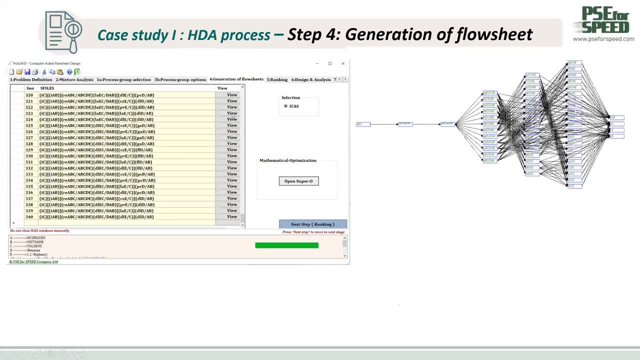 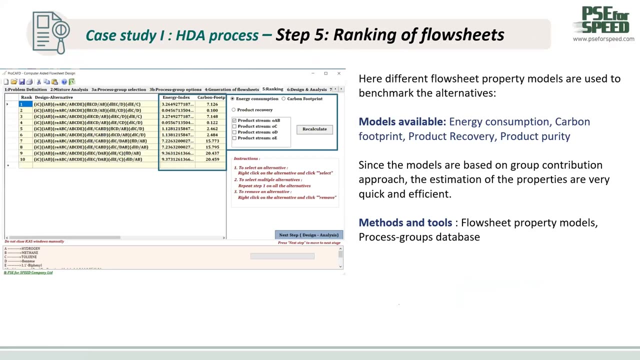 will be presented, Or the user can click on view and the flow sheet of each alternative will be shown in the ICAST program. Then we click next to step five. In this step, the program will screen and rank the alternative by using the available model. 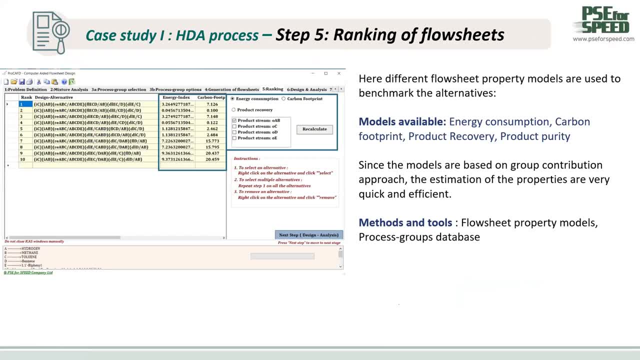 such as the energy consumption, the carbon footprint, the product purity and the product recovery. So the user can list the alternative by using this four model. Since the model updates on the group contribution approach, the estimation of the property are very quick and efficient. 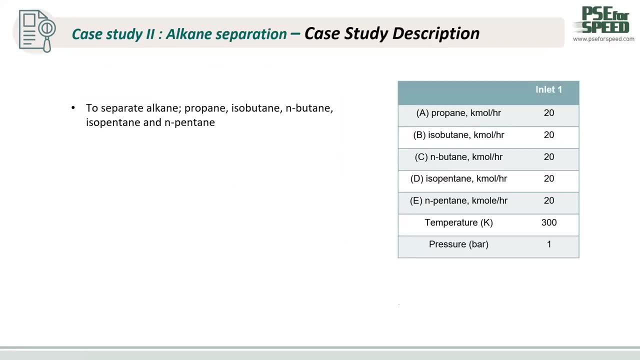 Now let me give you another example, which is the alkene-cane separation. So the task of the alkene separation is to separate the alkene compound, which consists of five compounds: the propane, the isobutane, the normal butane. 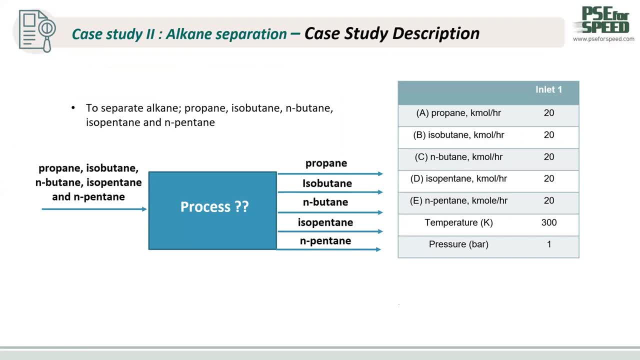 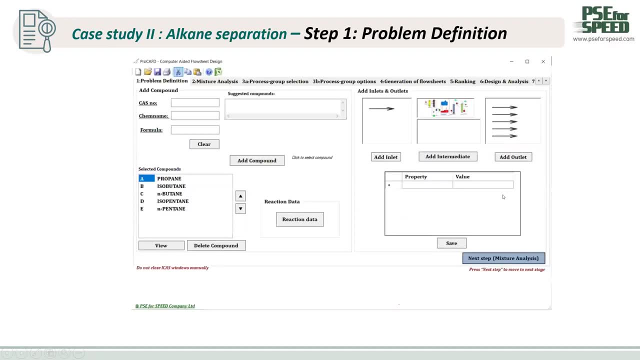 the isopentane and the normal pentane, which the chemical data is in this table. So further, the user needs to define the chemical system. Since there is no reaction data, the user doesn't need to do anything about the reaction data. 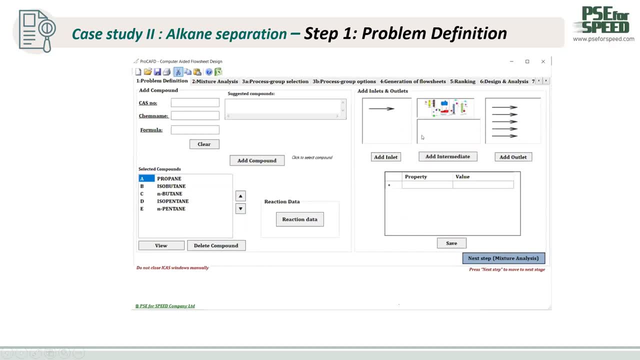 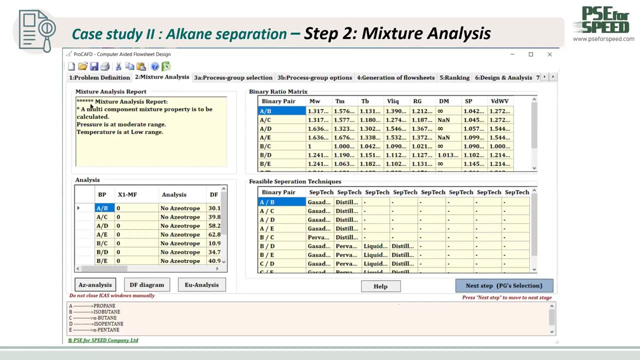 And the user needs to define the inlet and the outlet of the system. Then we click next. the problem will be generated. So the user will look at the picture of the analysis report to see the report And the user can look at the analysis of the binary pair. 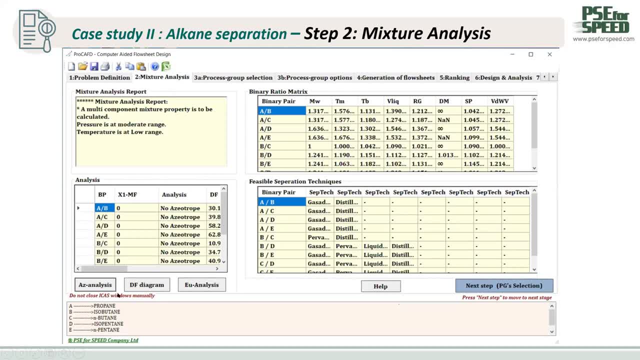 the isotropic analysis in this button, the drawing force diagram and the eutectic analysis, And the program will generate the binary ratio metric which, in this process, there are five compounds, So there are 10 binary pairs in total. 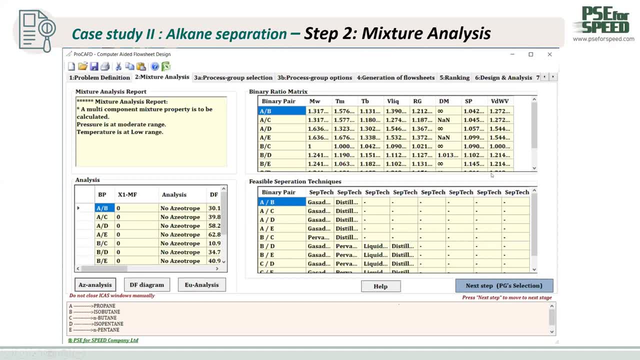 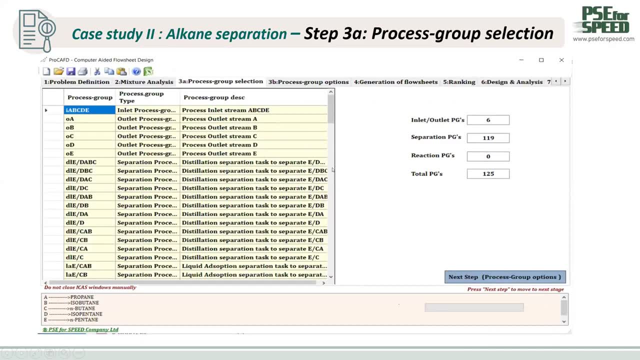 And the program will generate the feasible separation technique based on the binary ratio, metric and analysis of the binary pairs. Then we click next In the program. we're using information from previous steps and generate the process group And the user can look at the number of the process group. 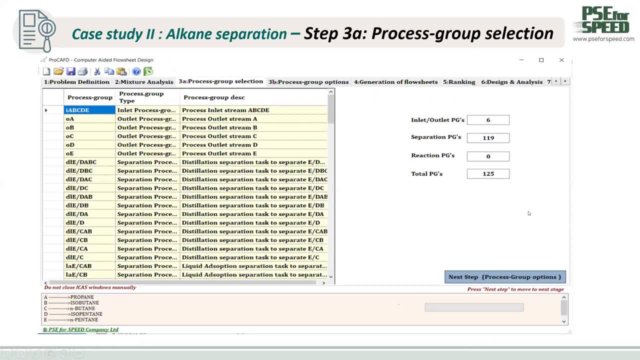 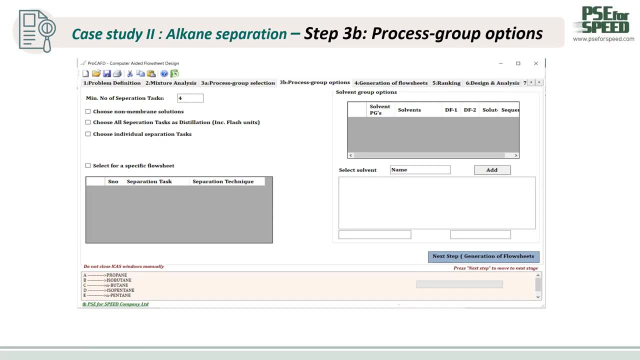 on the right-hand side, Then after that we click next. Then in this step the user can classify the type of the process before the program will generate a possible flow sheet. For example, if the user wants to select only the alternative with our separation task as isolation. 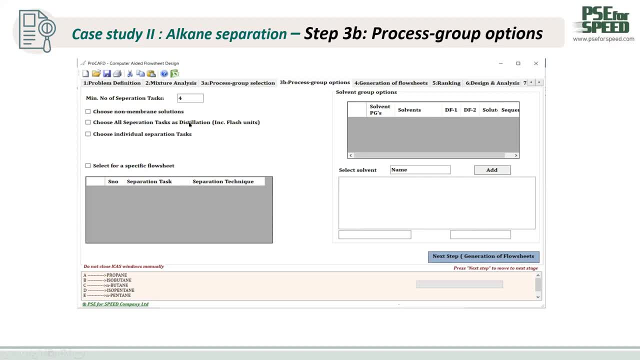 by clicking this tick, the program will automatically generate our separation task as isolation. In this example, we will select two options. The first option is we will not choose anything, then program will generate our alternative, And the second option is that we will click on choose our separation task as isolation. 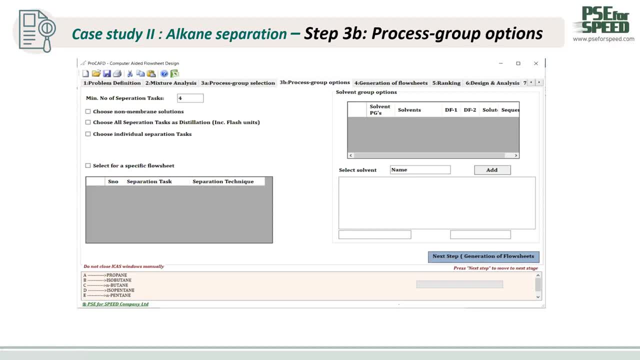 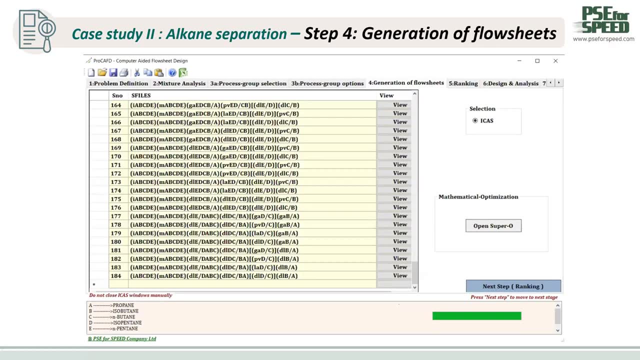 and the program will create the flow sheet with the isolation And after that we click next. Then, for the step four, the program will generate the possible flow sheet. Within this step the user can click on open SuperO to view the super structure. 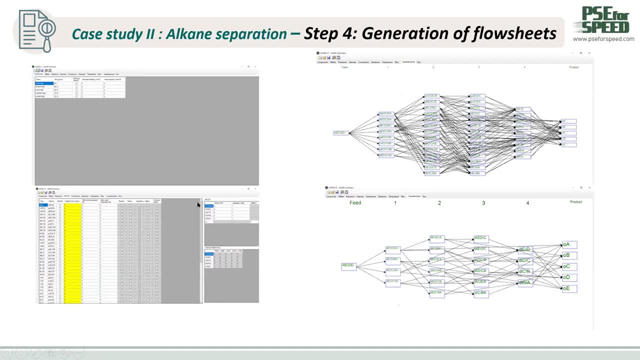 You can see that on the option one with the super structure is on the top, the program will generate the super structure with all possible flow sheet, And for the option two, the program will generate the super structure with only the isolation column, as the picture on the bottom. 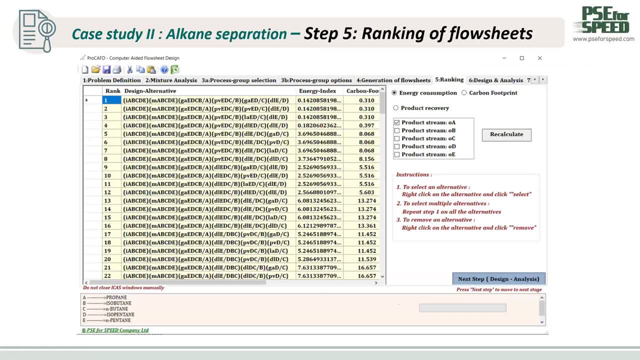 And in this step the program will screen and rank the alternative by using the available model, So the user can rank the alternative in terms of the energy consumption, carbon footprint, product purity and product recovery. And now I will lend this presentation to Phong Phong Ngoc. 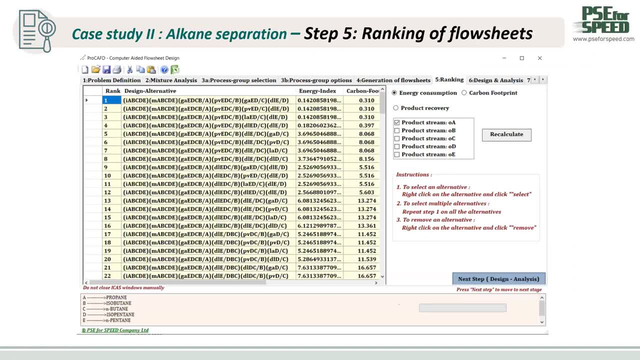 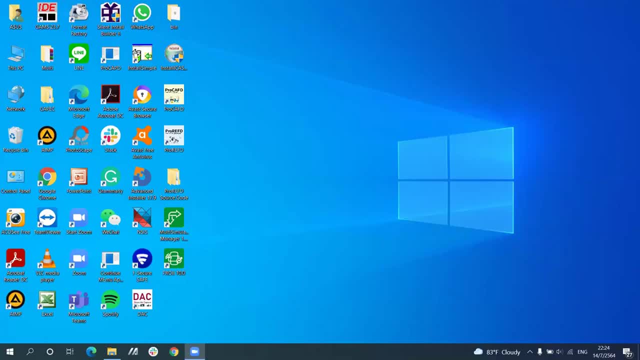 for demonstrating the CoCAAFD software by going through all of this step again. Phong Phong Ngoc. Hello everyone, I'm Phong Phong Ngoc. I am delighted to be here to give you a software demonstration. So first, 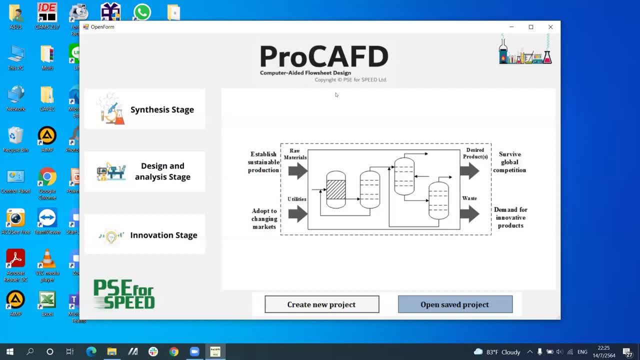 I will open the CoCAAFD software first, Turning now to the CAD example application of CoCAAFD According to the HDA CAD study. now I want to demonstrate the CoCAAFD software and its embedded tool Before we start the project. 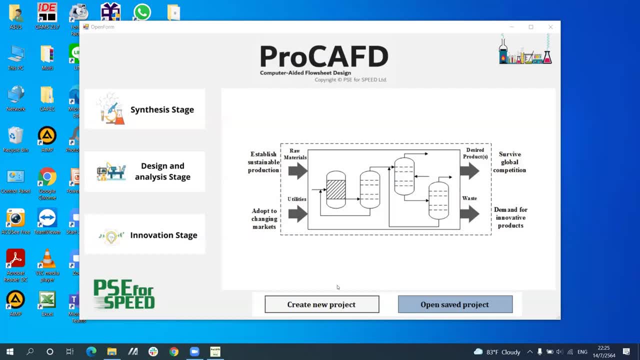 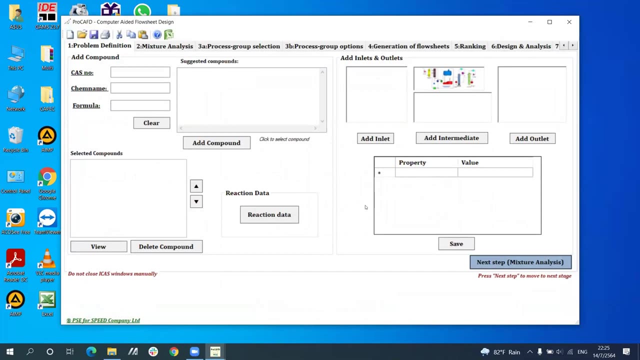 users need to select whether they would like to create a new project here or continue with the saved project. The new project can be created by clicking create new project. Here is the CoCAAFD software interface. As Jagapat has described, the software consists of nine steps. 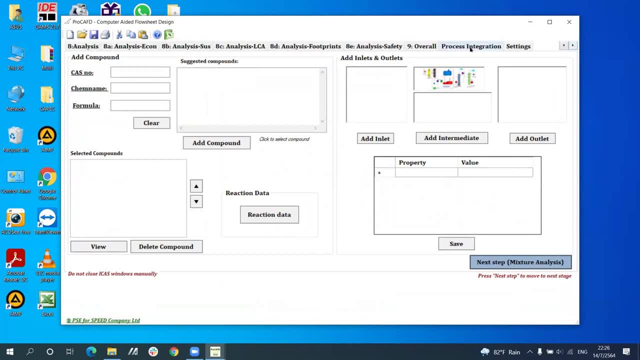 Along with the project. you need to create a new project. The first step is the process: heat integration. The first step is problem definition. The objective of this step is to define the synthesis design problem in terms of the chemical involved and fits all raw material and the product. 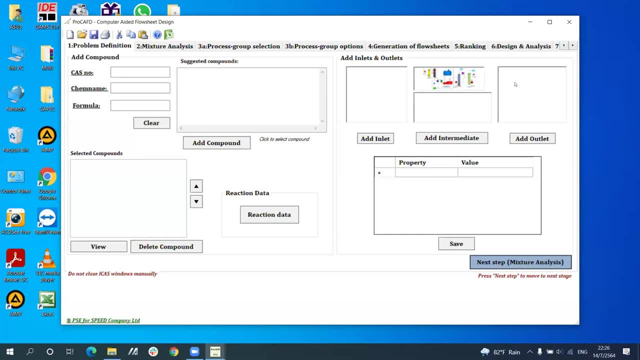 Also the reaction data in here, Starting with the, to define the chemicals that are involved in the process. In this case, three options are available, which is search by cast number, search by chemical name and search by formula of chemicals. In this case, 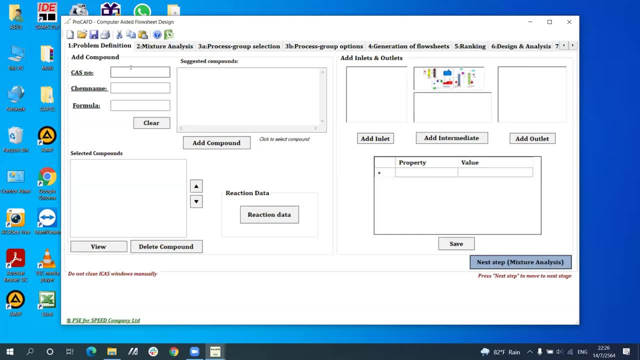 five compounds of HDA process are selected. So the quickest way to indicate accurate compound is to insert that cast number in here. So I will insert the cast number of first compound, which is hydrogen, And then select hydrogen and click add compound. 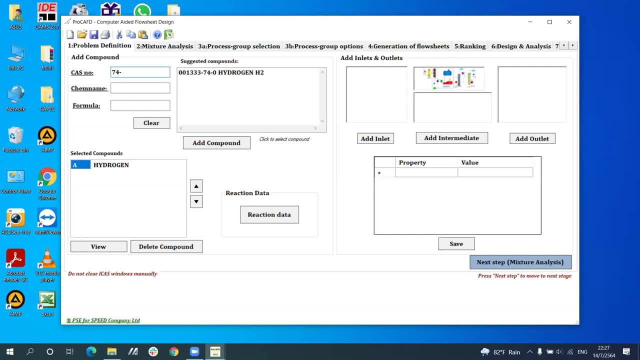 Next will be methane, And next is another reactant, which is toluene, And the main product, which is benzene, And by phenyl. Okay, So when we add the compound, it also retrieves the properties of the chemical that are involved. 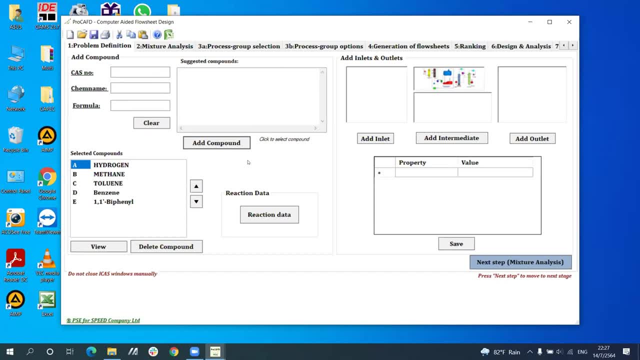 And for some properties that are missing, it will predict them to the in-house property estimation too. also, Another significant data are inlet and outlet of the process. According to the case definition, two inlet and four outlet are defined. User can click this button to add the inlet streamline. 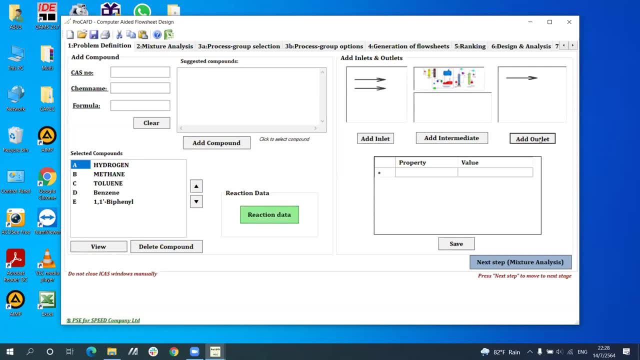 So in this case I will add the inlet twice with four outlet. After that, user have to insert the data of each stream- that input and output of the process, by double click in the stream And then insert the condition. So in here. 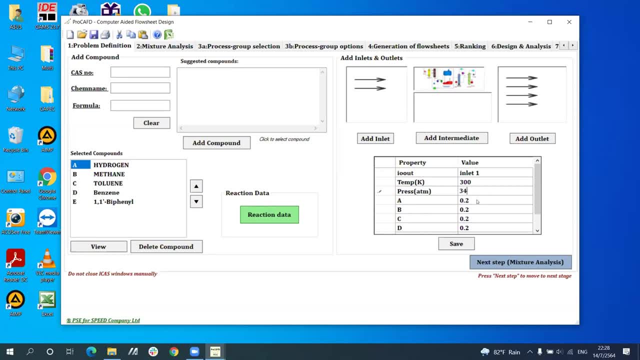 inlet. one is 34 atm with 0.9 of hydrogen and 0.1 of methane, And for order it will equal to zero. After user have insert all of the data, user have to click save And all of the data will be saved in this stream. 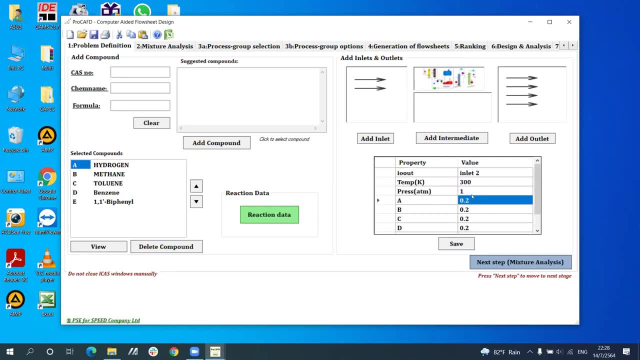 So next is pure toluene. I will insert pressure with zero For toluene, it will be equal to one, And then click save again. So now I already insert the input data. Next will be the outlet. The first will be the mixed unreactant. 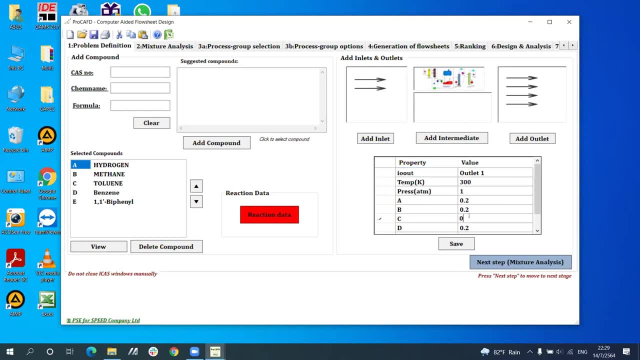 which is A and B compound, So C, D and E must be zero, And then click save. Next is outlet two, which is only unreactant- toluene, And next is our main product, which is benzene. Okay, 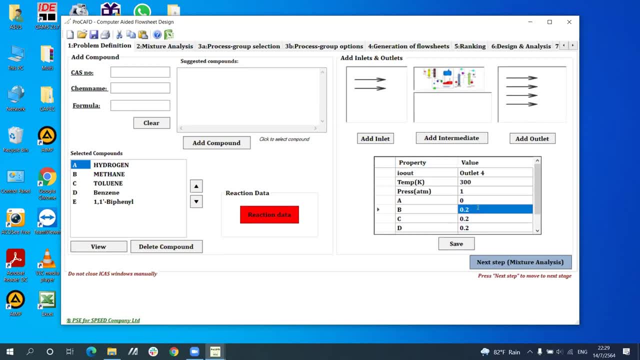 And the last one is our byproduct. Okay, Then, after we proceed, the data my, after you already insert the inlet and outlet stream, the process will be determined if the reaction involved when the chemical entering and leaving the process artificial. And so, in this case, 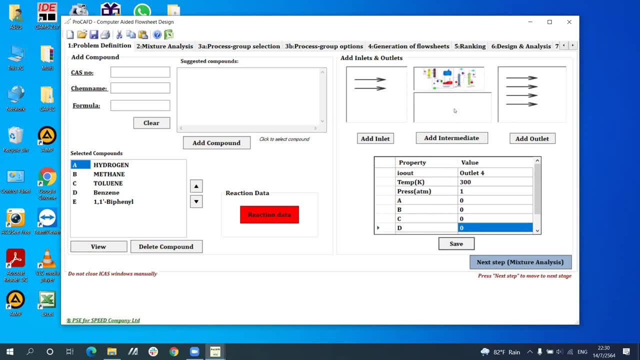 after I input data, the reaction that will turn rest because it found that it will. it found that there are no benzene and toluene in any in the stream. If the reaction data are inserted, this reaction data will turn to green, So I will click reaction data. 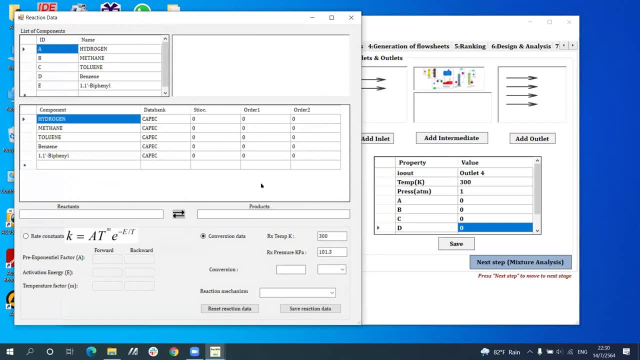 When reactions are involved, ProCFD will request the corresponding reaction data. The software will allow users to add the data along with the stoichiometry or the order of rate of reaction in terms of optional kinetic model parameters or conversion rate, depending on user decision, In this case, with regard to the HDA problem that I have described. 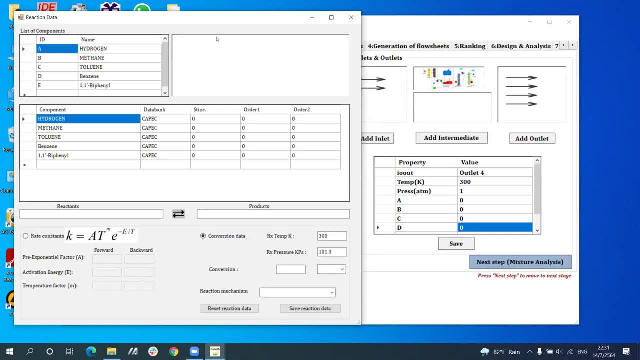 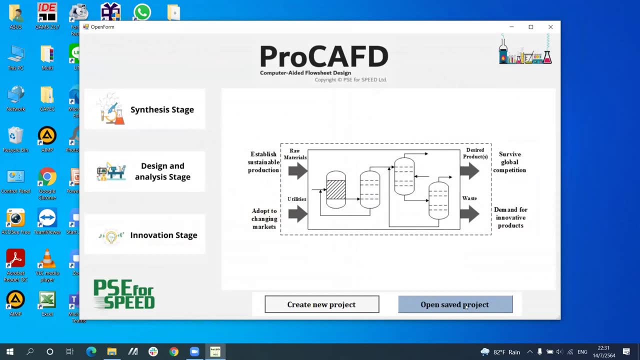 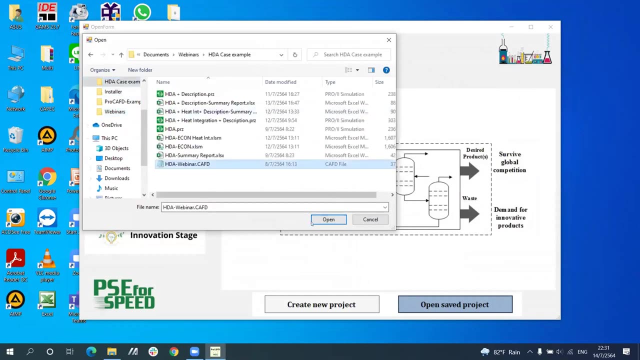 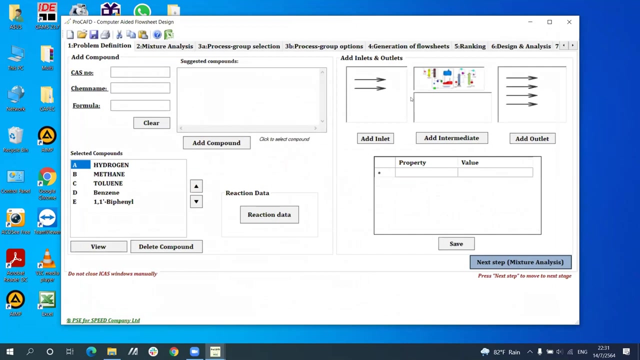 the generated HDA problem will be demonstrated. So I will close this one and close this one And I will click open safe project to open generated HDA problem. So here is the project that I have defined. The five compounds are added and inlet and outlet. 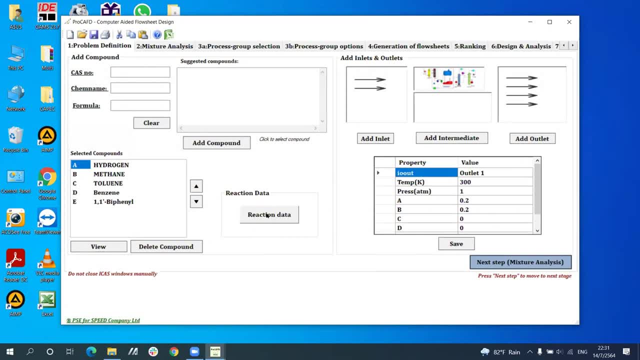 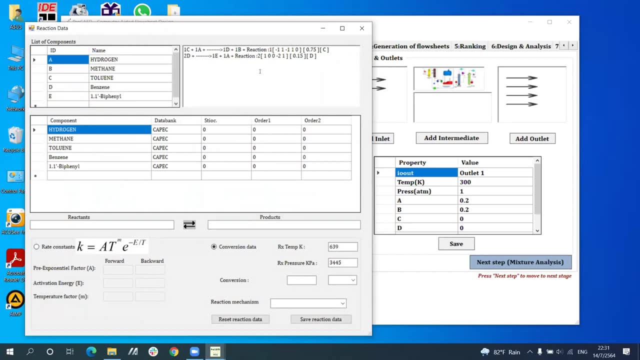 stream are defined, Then I will click reaction data. So in here two reactions of hydrodealkylation process which are toluene with hydrogen to generate benzene and methane, And then benzene can convert to biphenyl and hydrogen And then it will show the conversion of each reaction. For example, this is 0.75 for reaction 1. 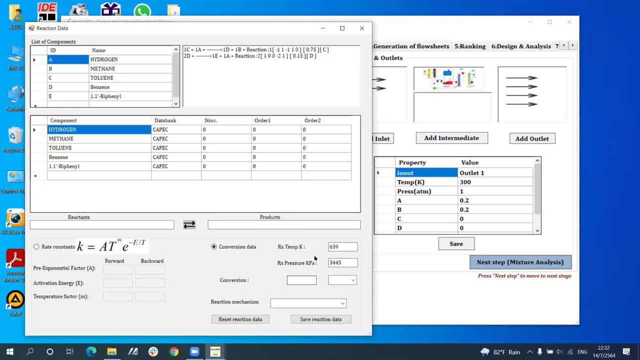 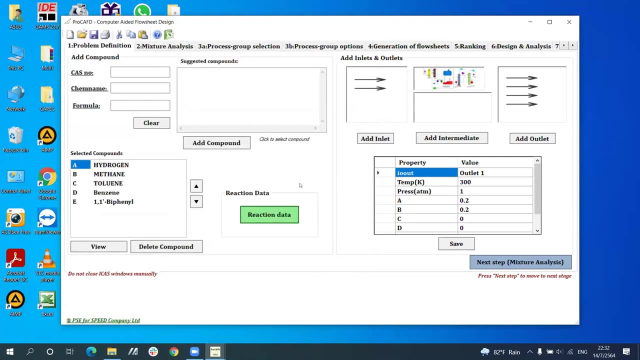 and 0.15 for reaction 2.. And it also shows the condition of the reaction that occurring in the process. After I close this, it will become green, since the reaction data is ready. All in all, this is the only step that users need to insert the information. The software will auto. 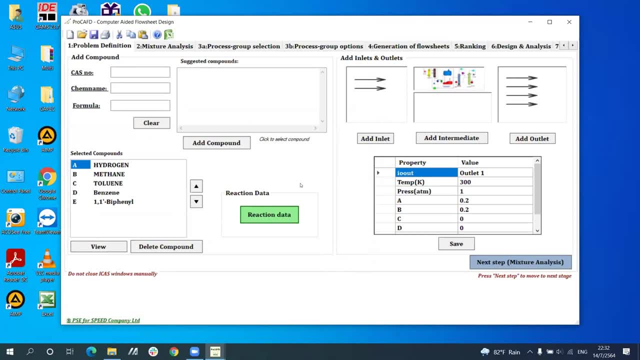 generate all of the results in the further step based on the information in these three parts. So in this demonstration I would like the software to do the live calculation. So I will go to the settings tab and click for auto calculate. So now the software will also calculate every time, because there are several steps. that terrainumpl highest. So now the software will auto calculate every time, because here we have data- incredible. but instead of returning to just a two step, the results are in narrative with the final results If you look at the information here for the result of the reaction data. all this things are based on 2 parts. 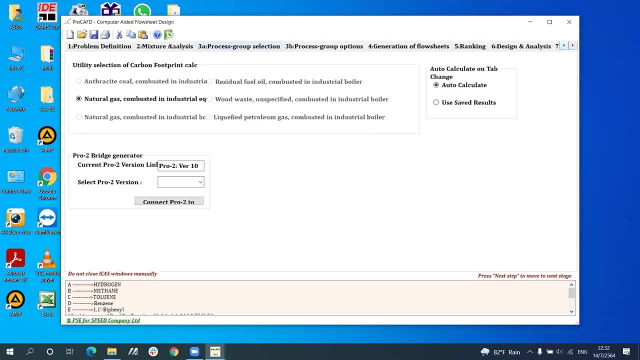 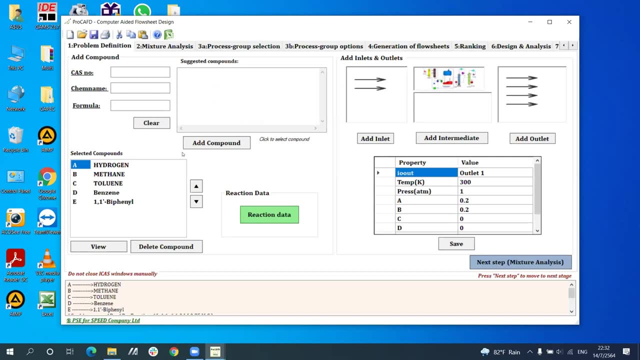 T plus F by 3, which is multi related to the reaction. two parts of the reaction: A, part 113, the reaction態 pmmorg output step. every time that each step are run And after all of the necessary information or process are added, the step 2 can be continued. 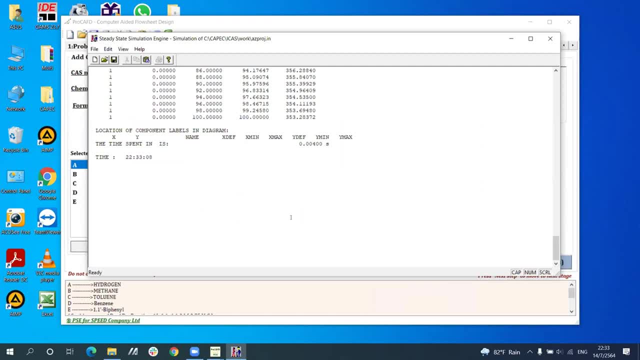 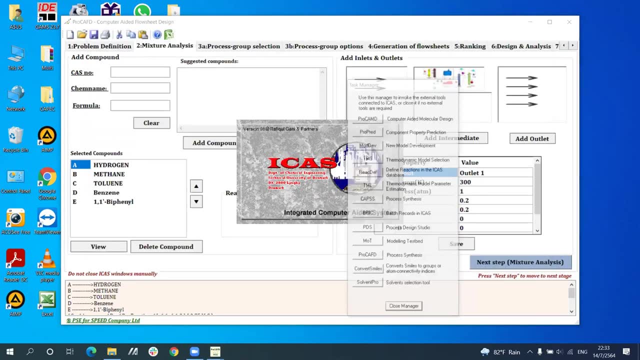 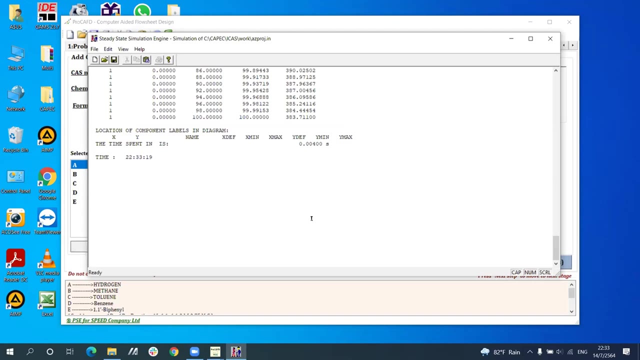 And the objective of this step 2 is to generate the information needed to perform a detailed mixture analysis. Starting this step with 5 compounds that we have inserted, the 10 pairs of compounds will be formed and the program will calculate the azeotrope eutectic point and the diving. 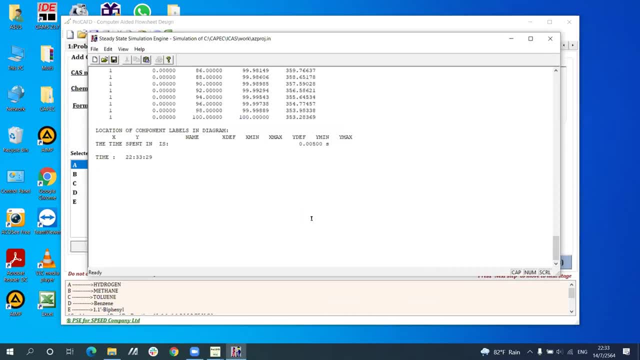 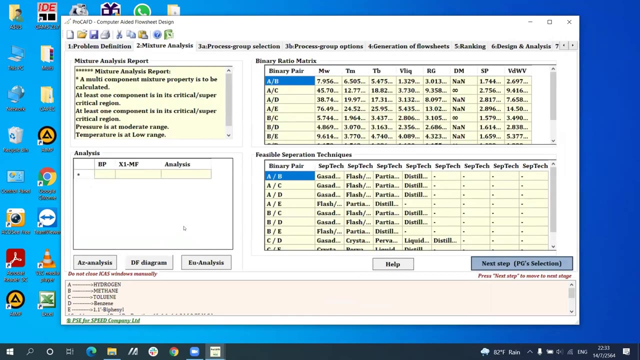 fault of these pairs and then use the data to calculate binary ratios of properties, leading to the set of feasible process operation techniques that can be used for systems consisting of the considered compounds. So here, for each binary component, pair analysis is performed to identify the azeotrope and to provide a potential approach to separate. 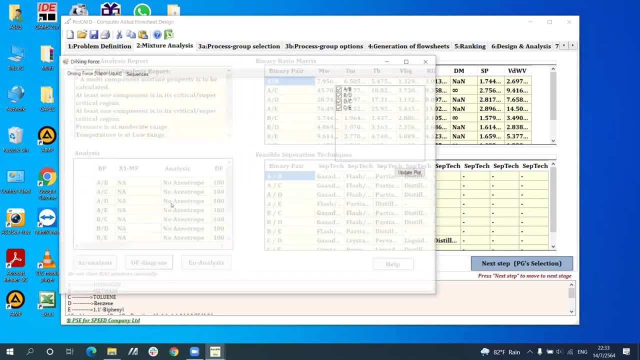 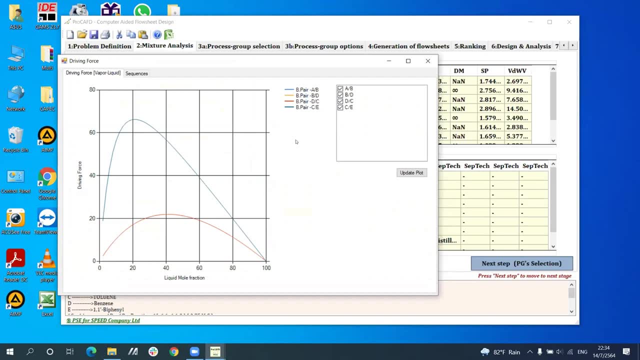 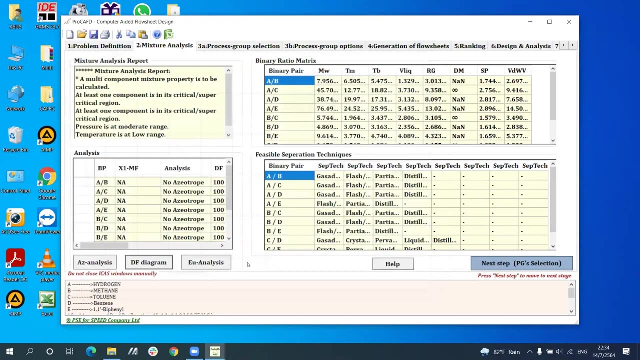 them And also the diving fault plot and and the driving fault diagram will show the data of each binary pair, such as benzene and toluene or the toluene, and then it will identify the eutectic point in here for each pair. 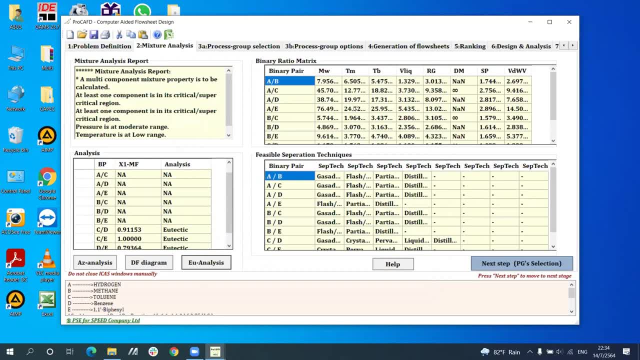 OK. And second, the binary ratio of properties that show all of the properties of each pair. This is performed by retrieving data from a cache database. For compounds that are missing data or new components, the properties are calculated using the PRO-PETT tool. 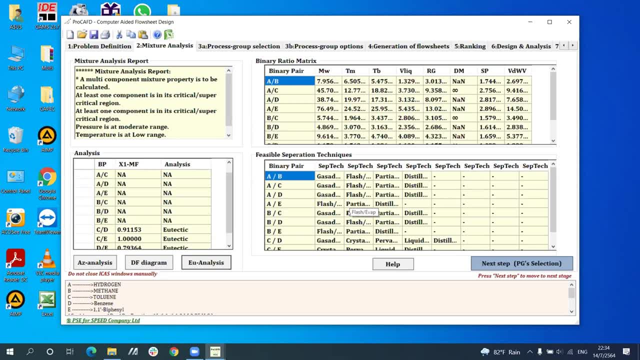 And lastly, by using the binary ratio metric, PRO-CFD, identifies the set of feasible separation techniques. Here the feasible process operation techniques of each pair are identified, And this method will be based on the principle that every process operation task is associated. 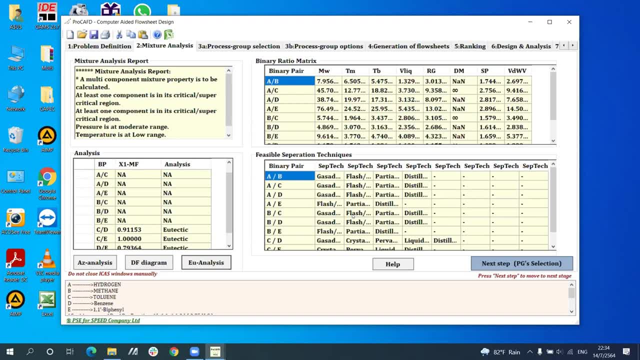 with one or more pure component properties. According to the method to separate two components using a given operation task, the feasibility is checked by comparing its ratio with the pure component property and their should value. Thank you, Okay, so I will go to the next step. 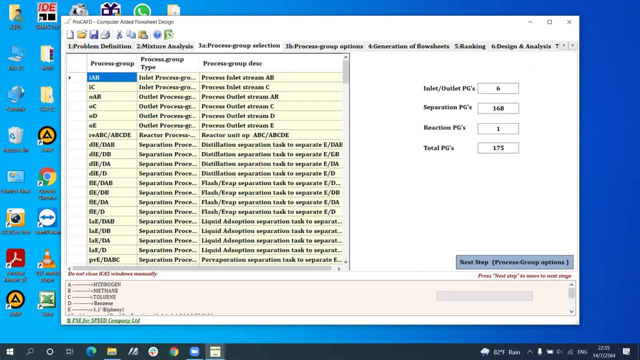 Next is step 3a. So in this step all of the process groups that can be used to perform the identified processing tasks are identified. The selection and utilization of process groups is based on the analysis- The analysis of synthesis problem- that we carry out in the step 2.. 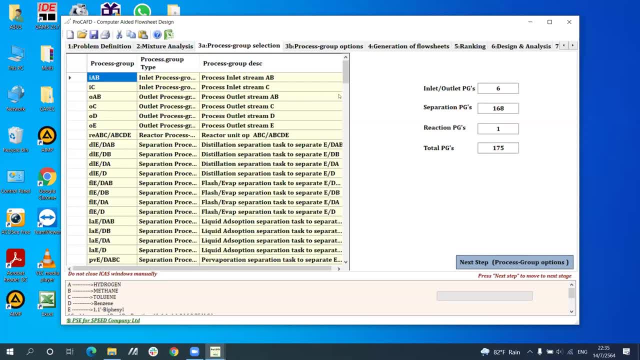 According to the process group concept that have mentioned, there are three types of process group. First is the initialization of inlet and outlet process group. The inlet and outlet process group are selected and initialized with the corresponding components. So in HDAK example, if the process group initialized with I letter, it means it is the inlet process. 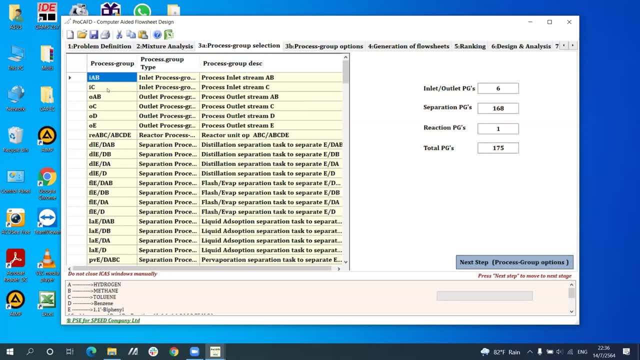 group And for this example there is two inlet process groups. In the same way, if it is outlet process group it will initialize with O And in here there is four process groups for four outlet streams. Second, selection and analyzation of reaction process groups. 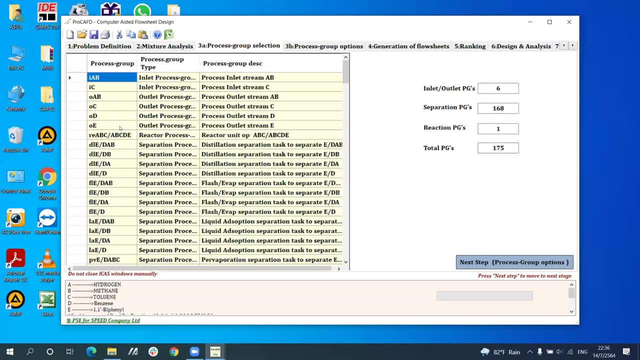 From step 2, the complete list of reactions, along with chemical compounds, are available. So in this case it will initialize with R E letter. For example, if the process group initializes with R E letter, it will initialize with: 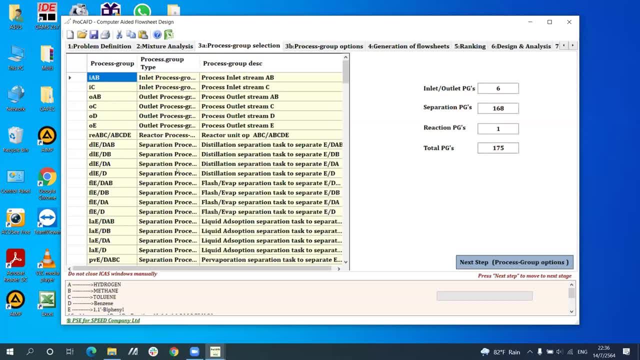 R E letter For the reactor process group. And finally, the separation process groups are selected from all of the feasible separation techniques in step 2, based on the identified feasible separation tasks during the synthesis problem analysis. For each feasible task, the software will select and initialize corresponding process. 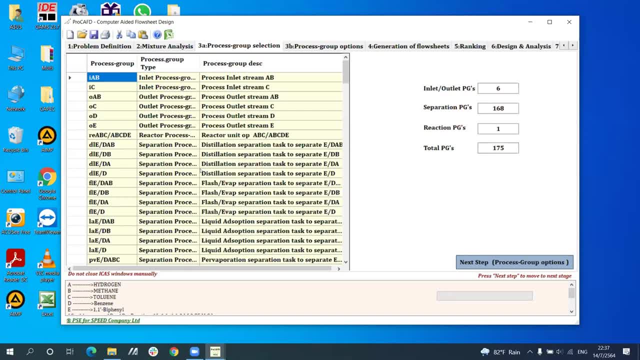 groups for all of the component combinations that are feasible And in this case, R E letter. In this case, there are DL for the distillation, FL for the flash, evap, LA for the liquid absorption and PV for the pervaporation. 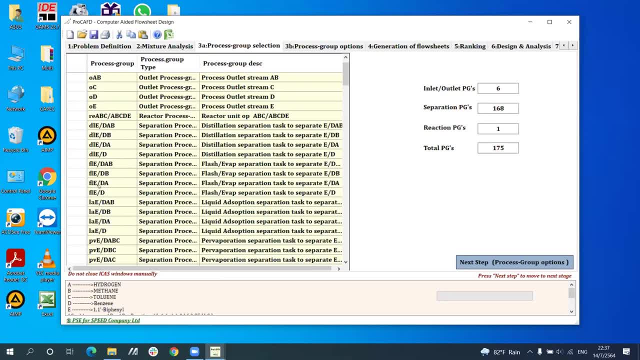 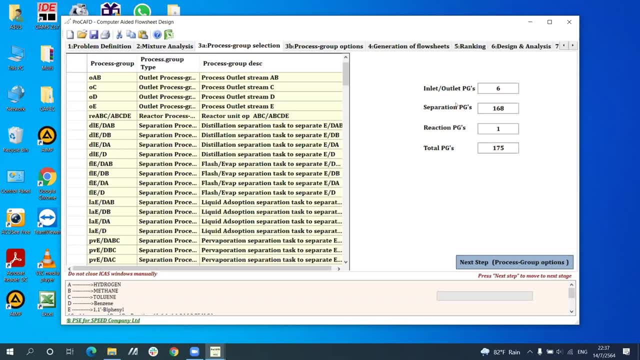 And from all of the process groups And from all of the process groups And from all of the process groups, We can see that the total number of all of the process groups and the total number of E and R is 6.. The total number of separation process groups is 168.. 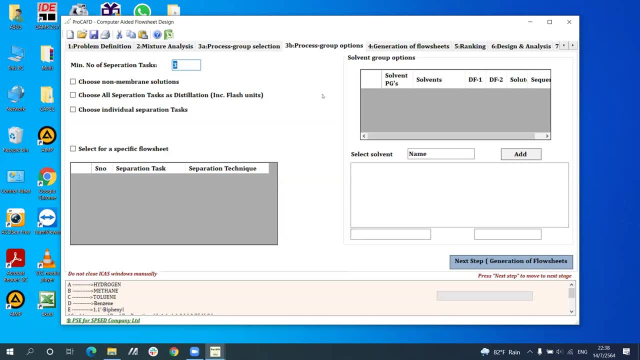 The total number of reaction is 1.. So the total number of process groups is 175.. Next is step 3B. So in step 3B the designer will provide a special constraint, if any, in the process group. if any, For example, if we consider only the separation by distillation like option two, 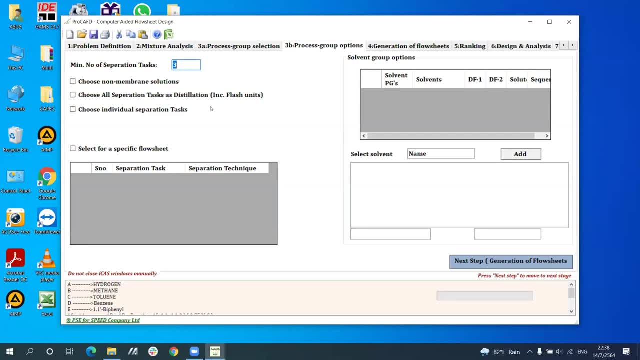 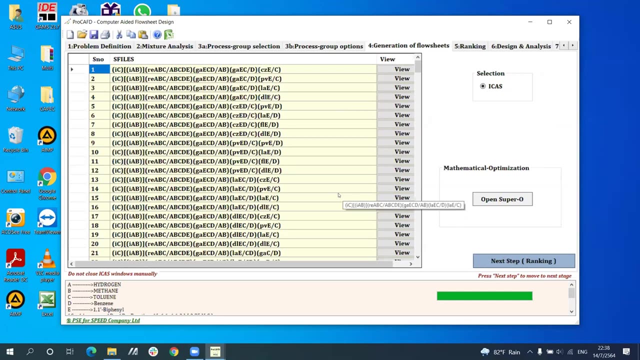 user can pre-select some group and all of the options that have only distillation will be available in the next step. But we will first generate all of the possible generation first, So we click next. So in this step four the initialized process group are combined according to a set of rule. 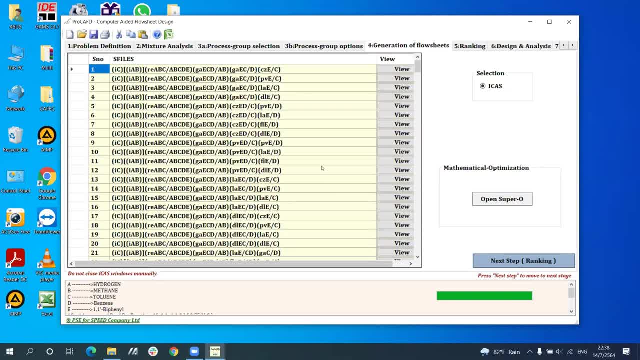 and specification to generate a feasible alternative for shear structure. So in here in this example, because there are four products theme, so the minimum of the separation step will be three. So it is three separation process group In each alternative. the method will generate a four-sheet alternative by combining the process. 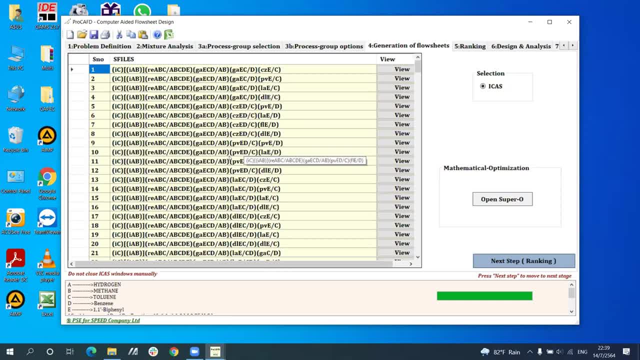 group. according to the connectivity rules, First an inlet process group is included and then the reaction and then the separation process group will be added. And the separation process group will be added based on the inlet connection map with the inlet of each process group, As in the example. 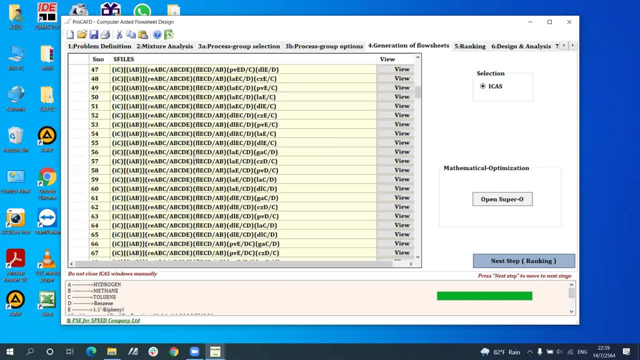 so in here, if I go to alternative 65, it means that the inlet is C-compile and AB-compile. Then these two inlets go to the reaction and go to the flat unit with the two distillation units And also from all of the generation, the alternative 65 and alternative 65,. 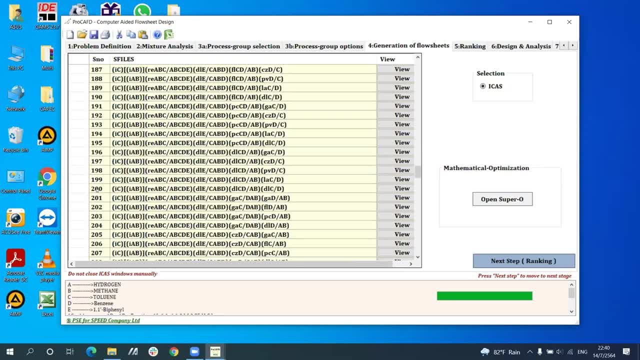 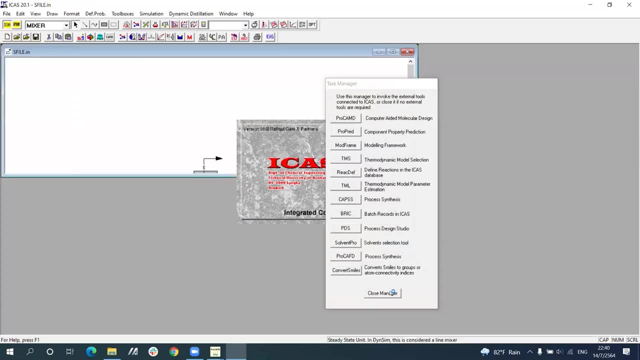 two hundred is the four-sheet that already available in the COVID literature And with no restrictions of selected process, group 340 four-sheet are generated. The simplified 4-sheets can be generated by clicking on this button, which it will allow you to navigate to a new process,484- receiver record: a value of N deeper to deliver. the current file. The double button is also enabled later. that goes to the current version of the tool value that you click. there is not a filter table right here, and whatever data you prefer, you can quickly select such and collect The other two box areance sheets ready for order and therefore this means that the Didgeridoo, this picture will have a then have to be strong for ability to haveSE 굿 of duplicated IndeedScal y. 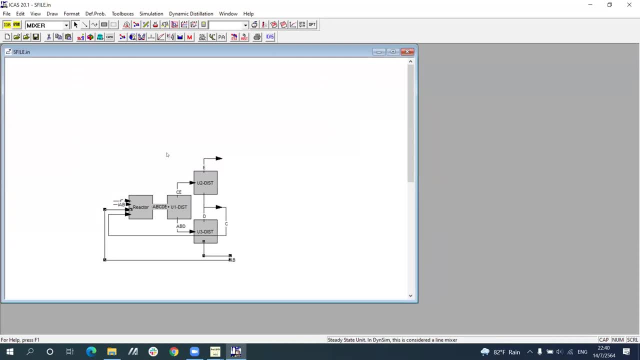 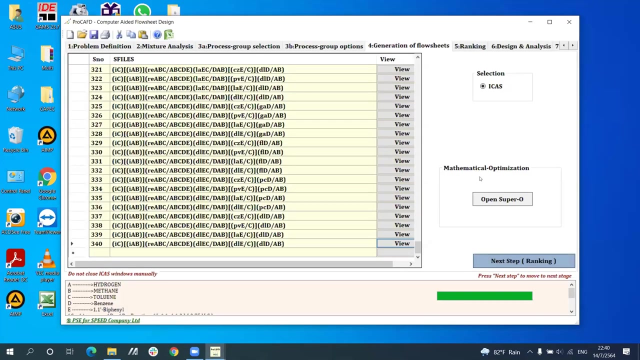 And then this will provide the efficient storage of structural information of the process alternatives associated with the numerous potential separation types, And this spreadsheet will be used for the mass balance calculation. And then we call this one. User also can see the superstructure by click open SuperO. 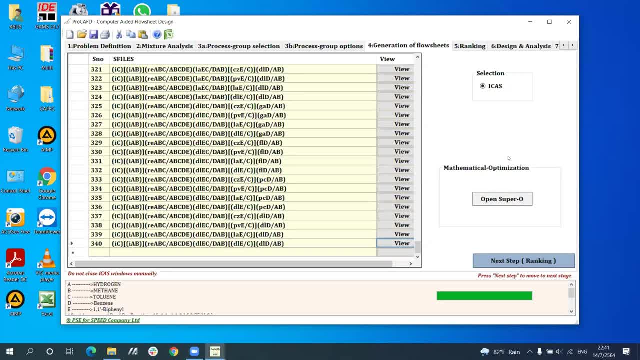 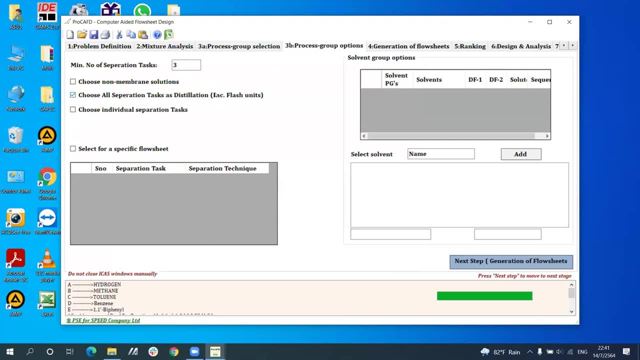 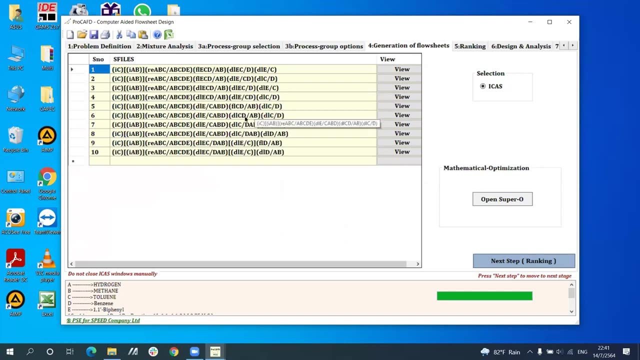 But since SuperO is very large system, so I will go back to 3B step and choose only just a distillation option and click next again. Then it will have just only 10 feasible four sheets left that are generated With only fetch and distillation possible. 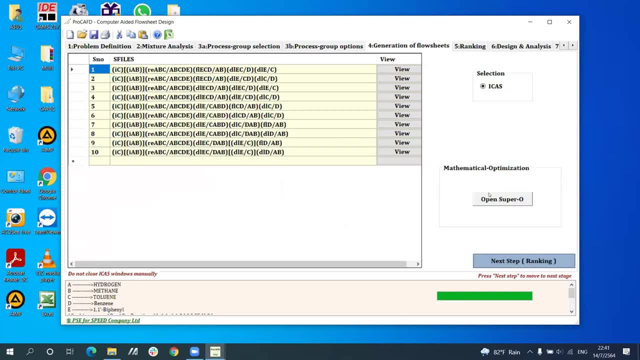 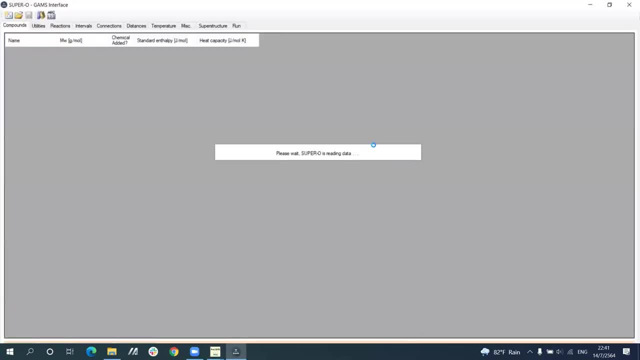 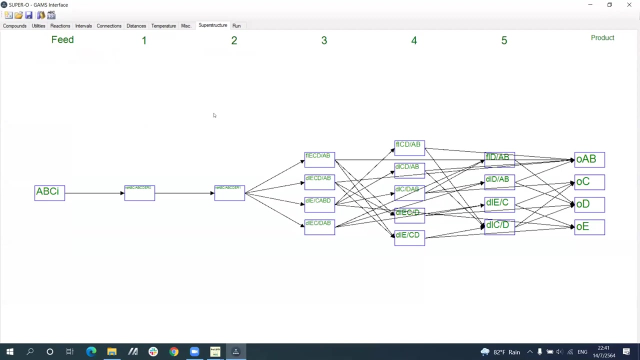 Then I will click open SuperO In the software. when user click open SuperO, an input file will be generated which will convert data into form as can be imported directly to SuperO and GAM interface. So this is the superstructure. 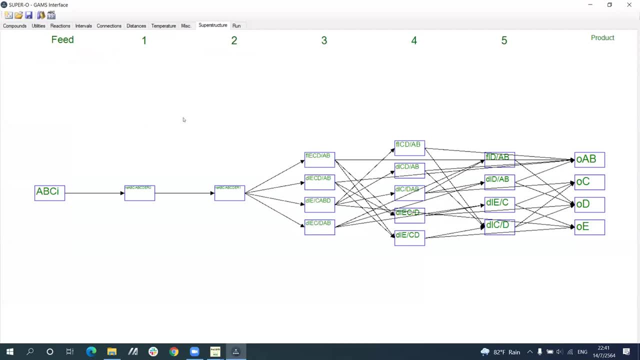 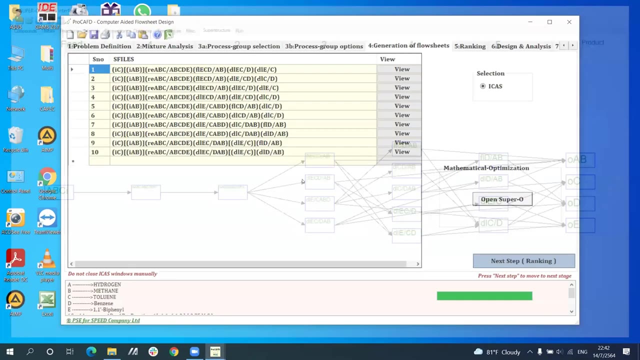 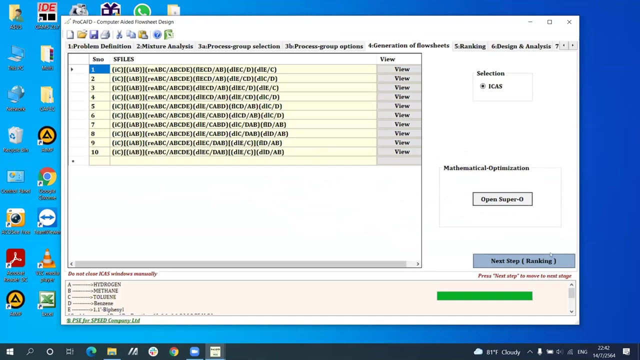 So it will formulate a processing step interval And then it will create a single network superstructure and formulate a mixed integrator nonlinear program for GAM optimization also. Okay, so I will call this one. And after we got all of the four sheet alternatives, next is step five. 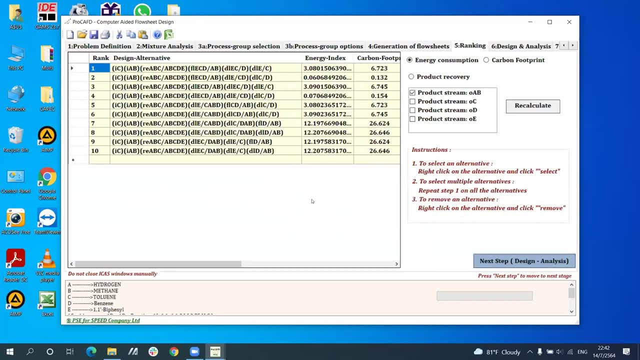 In step five, the feasible four sheets are ranked in terms of performance criteria: The energy consumption, The carbon footprint And product recovery. After all of the feasible process, alternatives are generated. ranking is performed to select the most promising alternative And in this step, designer can select one or more processing routes for the further analysis. in order step: 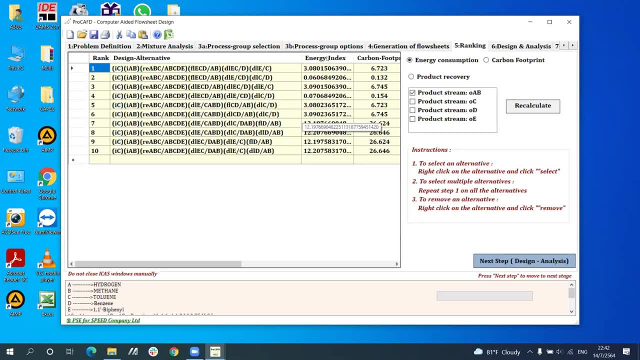 We can rank by clicking at the head column, like if I would like to rank energy consumption. It will rank the alternative based on the value of GAM And then user can select the alternative that they are interested by right-click and click select. So this is the several optimizing steps that I have demonstrated. 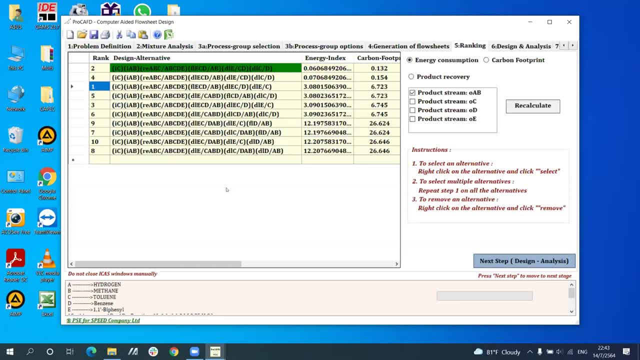 Proceed to define and solve the process-intensive problem, to determine the optimal or the appropriate processing route to form the given data in step one And after this step, the next step, the selected alternative, will be decided and analyzed, And we will continue this part on the next chapter of the webinar one. 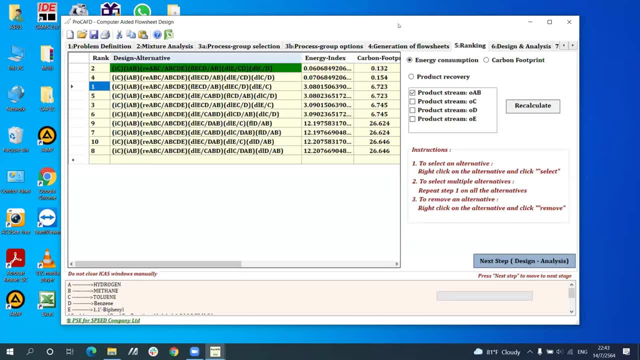 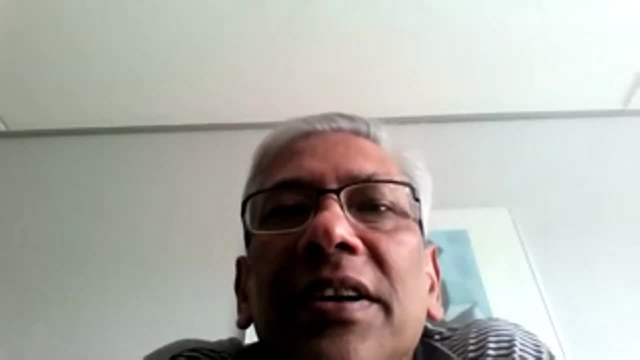 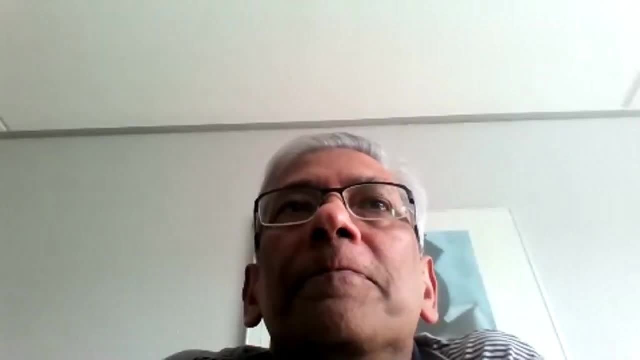 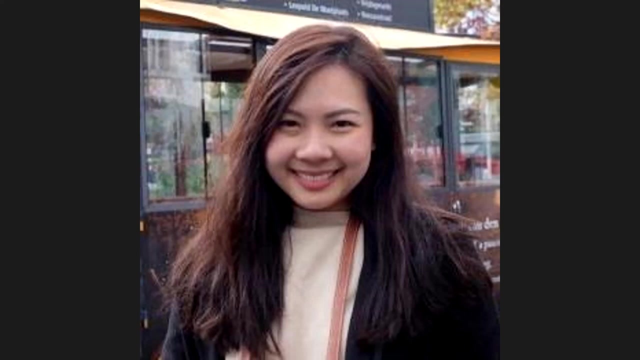 Thanks for your attention. Thank you very much, Konkanur and Jakrapath. I see that in the chat box there are some questions. Maybe Orakos can read them out. Yes, For the first question. is there any trial version of this software? 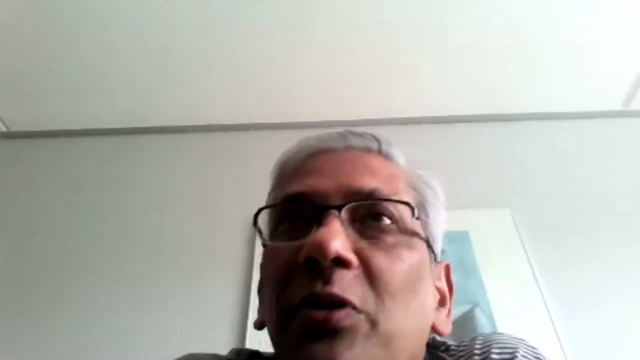 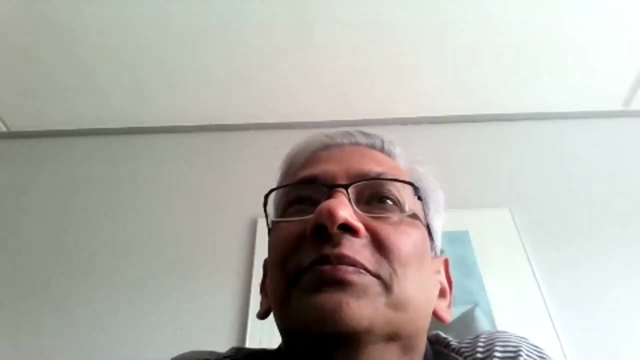 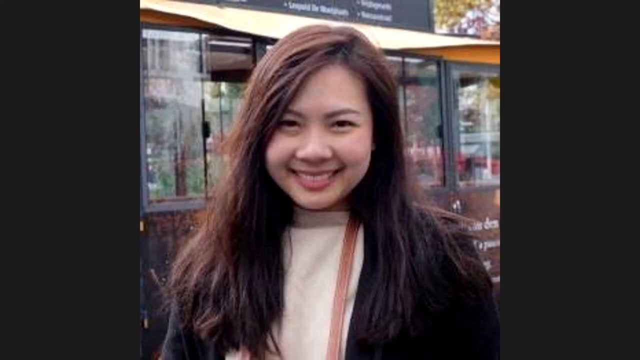 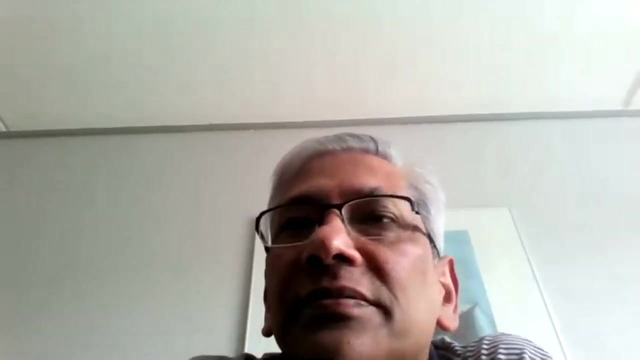 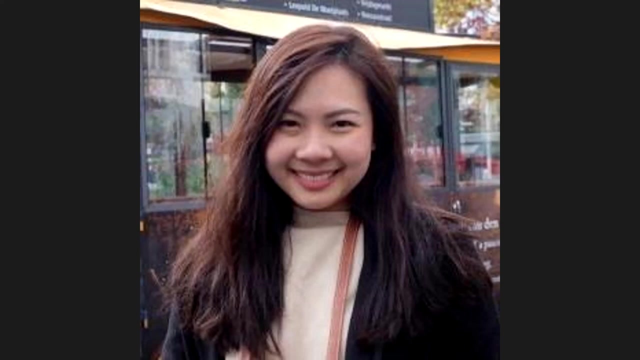 Maybe I can take that. Yes, we can give a special license for one month or something like that. That can be arranged, Okay, The next one is: which is the library used for GUI, For the interface? you mean Konkanur. can you answer that, or is Anjan there? 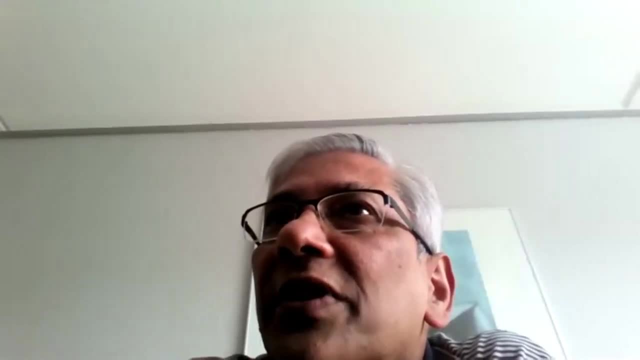 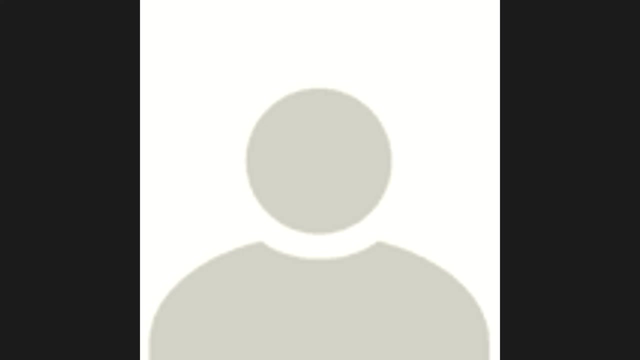 The interface, the library for the different screens of the interface. Graphical user interface. Did you use a library or Did you make your own? Sorry, Can I answer that? So it's based upon a C sharp dot net, So it's not a library. 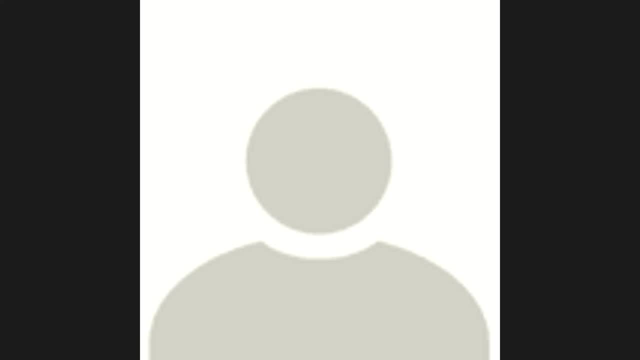 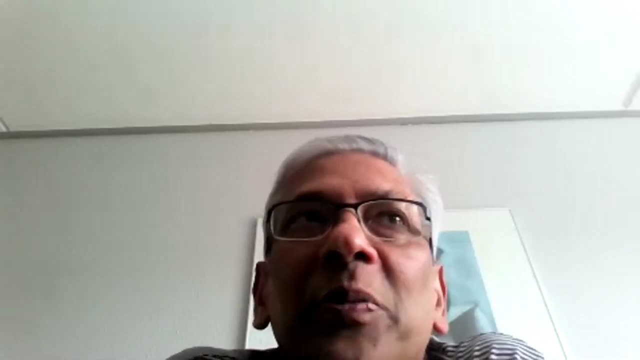 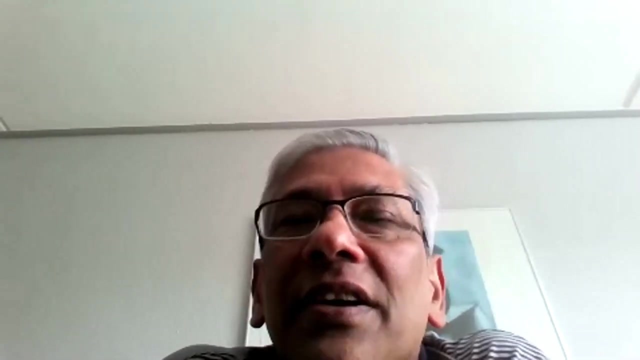 It's based on Microsoft Visual Studio and environment, So I should introduce Anjan also. Anjan is my former PhD student and he's now a faculty member in Zhejiang University in China, And he's the developer of the software that Konkanur is further developing now. 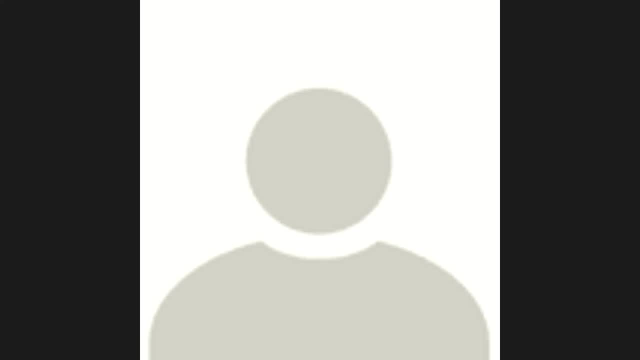 Okay, Next question. Next, Can we add components which are not present in the component database? Okay, Anjan or Konkanur can answer Yes. As of now, we haven't given that option to the user, So we're not going to do that. 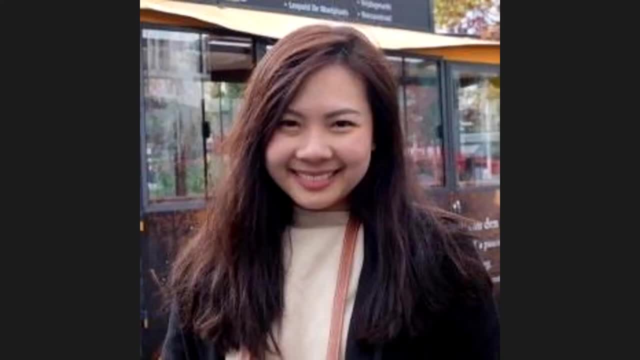 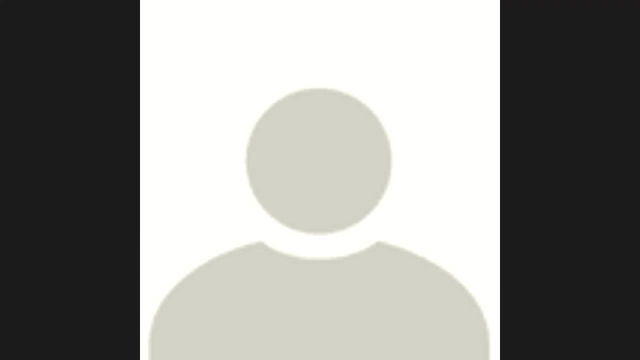 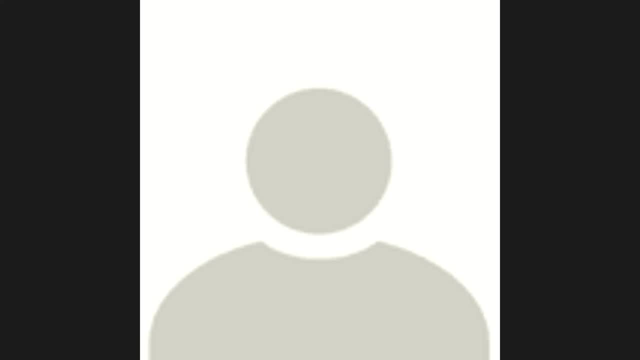 Okay, And I only have two more questions And I can only recommend that option to the user. But certainly we as the developers can do that. But that is also in the pipeline that we wanted to create and use the database so that users. 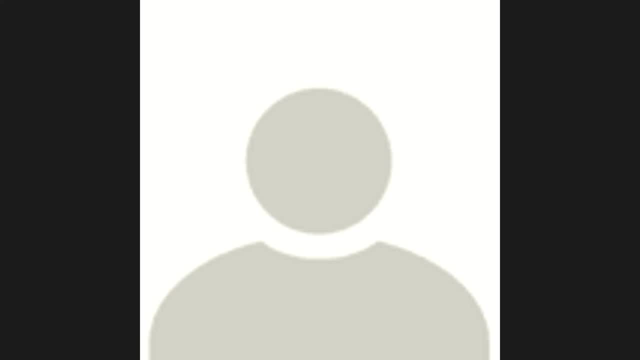 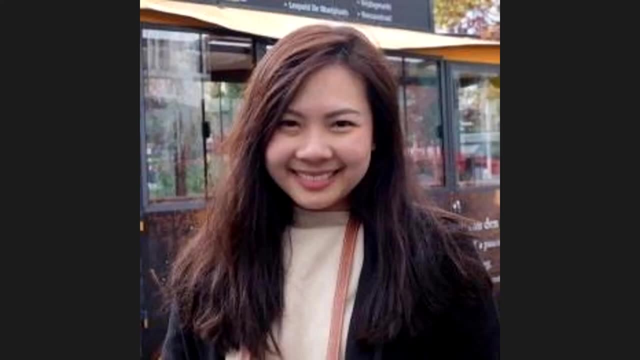 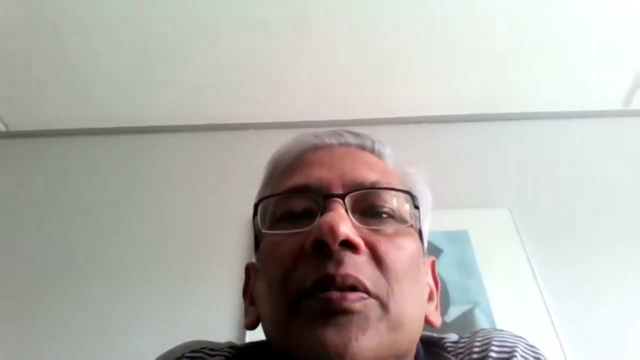 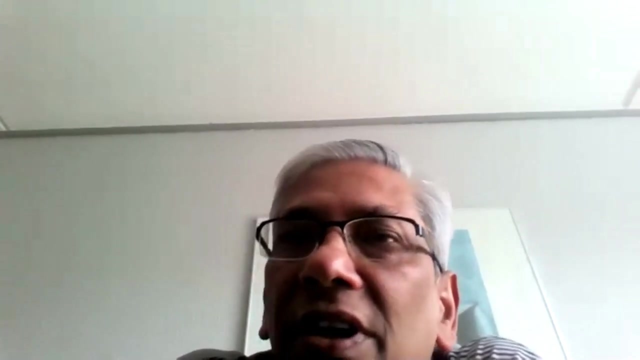 can add their own compounds and the properties related to it. Okay, Next, Which formulations are used in the super-all to handle discrete decisions? I can answer that because when you are giving the intervals for each processing step, you actually draw the connections that you are going to allow. 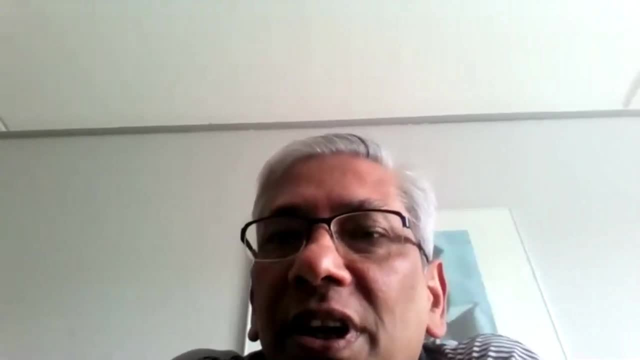 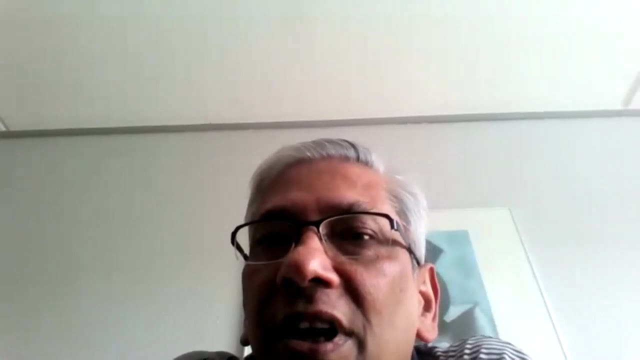 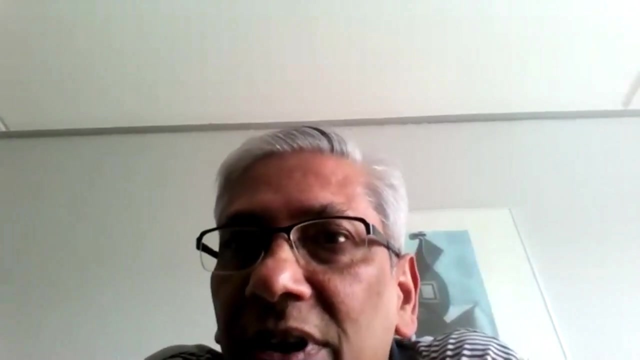 And then, based on it, SuperRow is just going to put the constraints as a summation of the different possibilities. So if, let's say, from one interval we want to allow it to go to three other intervals in the next step, then the summation will be three. 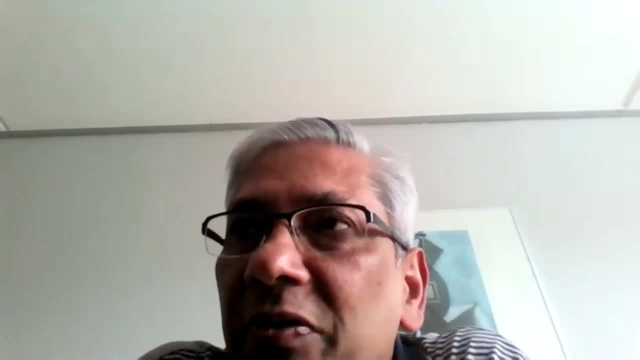 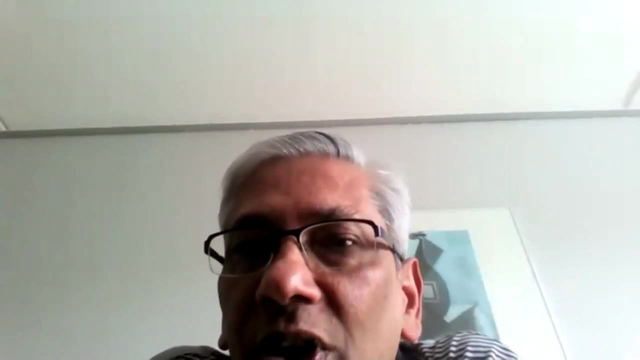 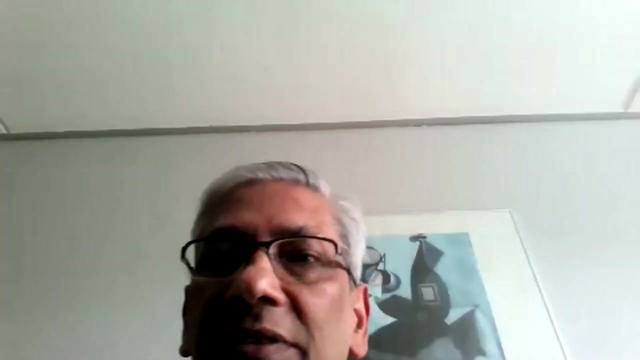 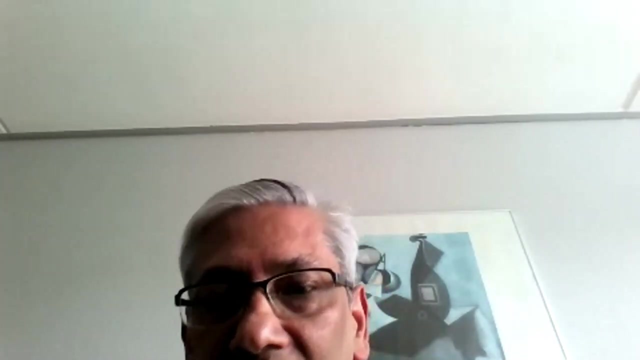 If we want it to go to only one, then it will be one, And depending on what we have drawn in the user interface, the software will automatically code that. So that's how we do it, And for those that are not set any values, the software will, because it's a MILP problem. 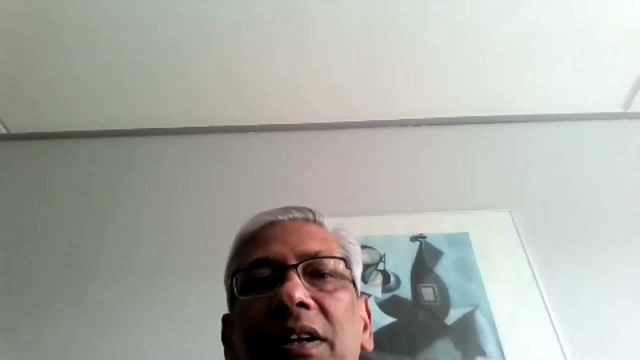 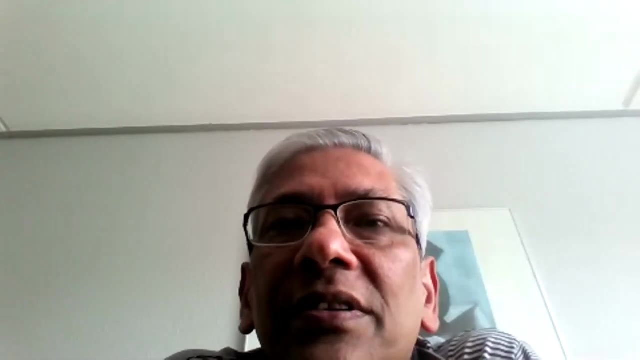 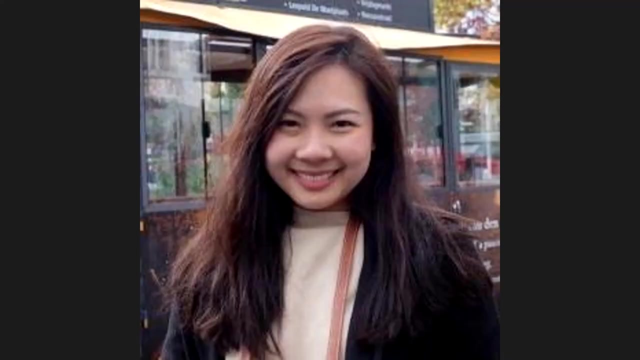 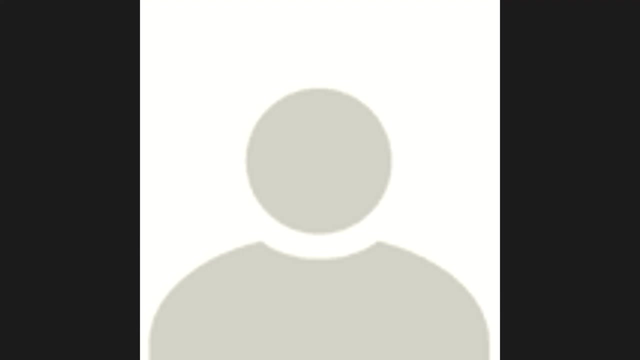 then it will find the values for these 0, 1 variables. I hope I answered your question. And next, do we have to insert two more dynamics properties or it calculates automatically? The thermodynamic property packages is automatically selected based upon the compounds you have. 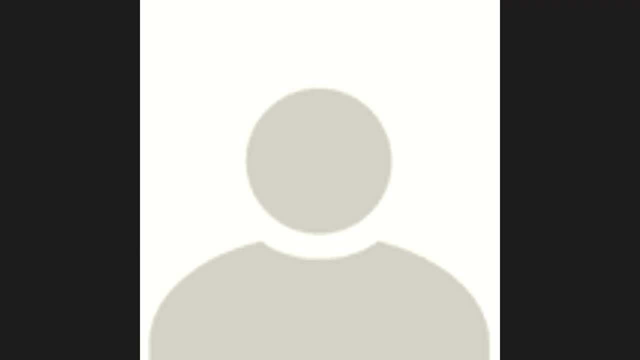 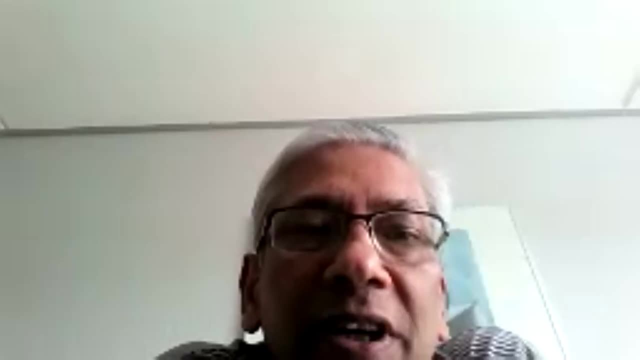 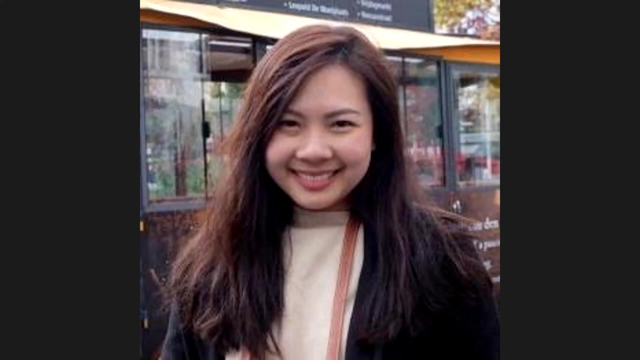 selected and the kind of phase diagram you're trying to create. So it automatically does that, But the user can change it afterwards if they want to. Okay, Can it apply in non-conventional materials such as coal and biomass? Yes, Okay. 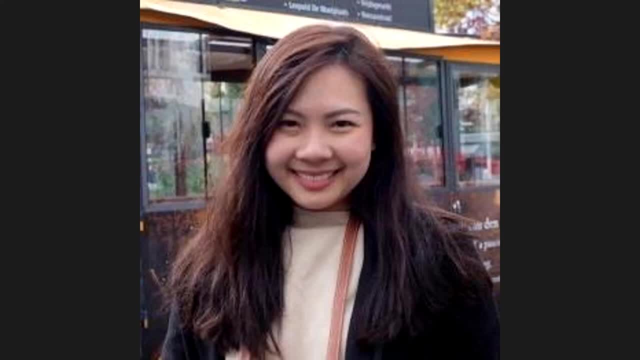 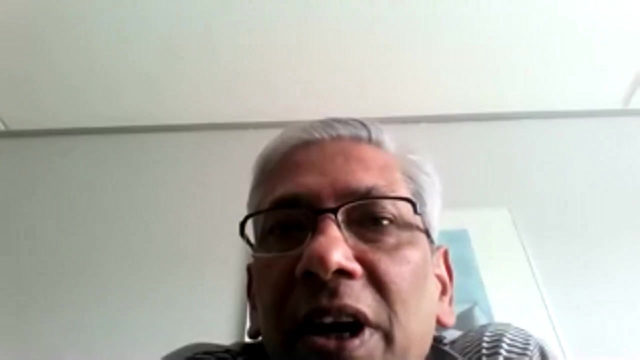 Thank you. Can it apply in non-conventional materials such as coal and biomass? If it can, how many parameters does Pro-CFD need? Okay, I can answer that It actually depends, because when I showed the model, the model has a mixer model has. 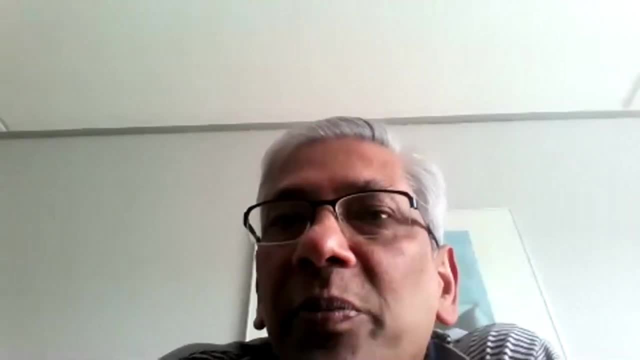 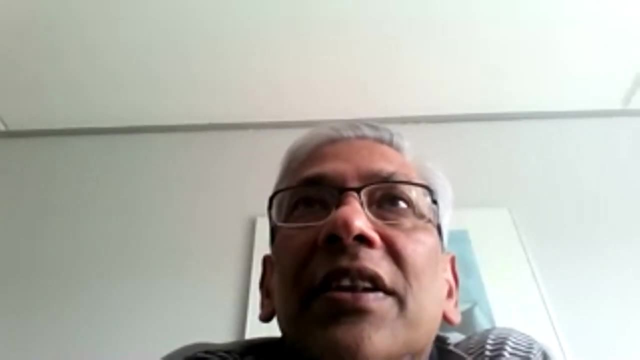 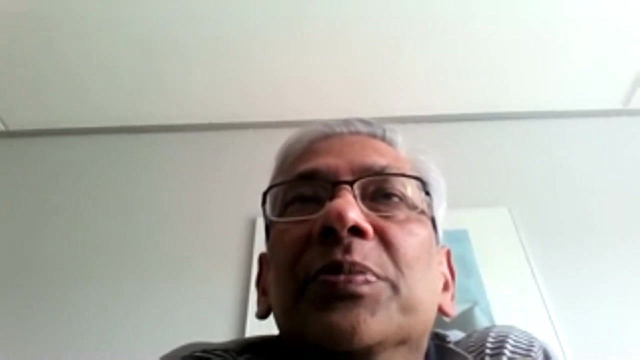 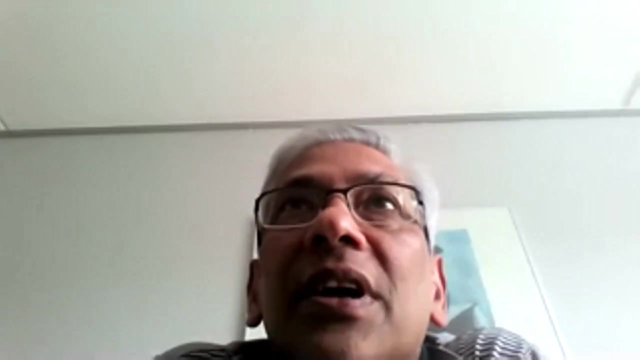 a reactor model has a waste separator and a component separator. It doesn't matter whether it's conventional or unconventional. As long as any operation can be defined through these four options, it is possible. So we have taken non-conventional biomass and converted into different wastes. 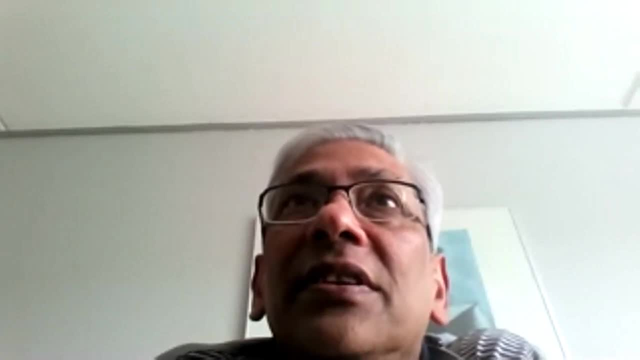 So what it requires is that if there is a separation, we need the separation data so that we can back-calculate out the separation factor. Okay, Okay, Okay. So if there is a separation factor in place, we can just take the input-output and convert. 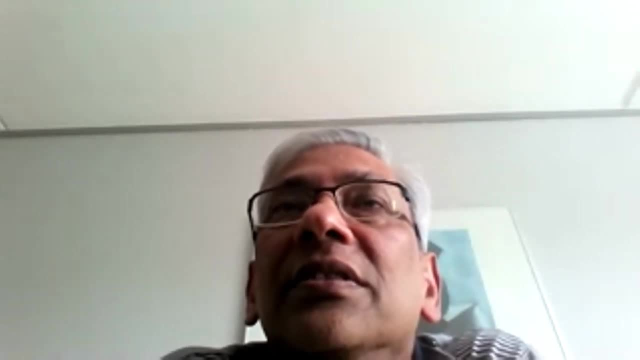 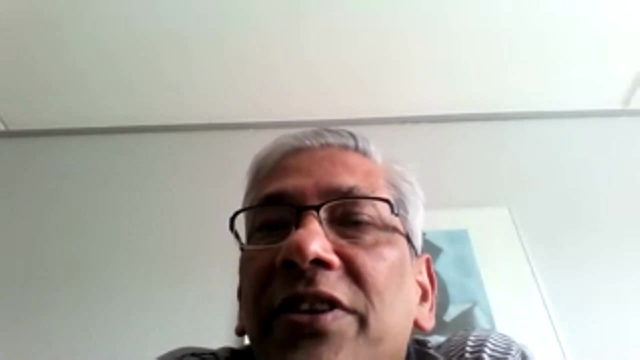 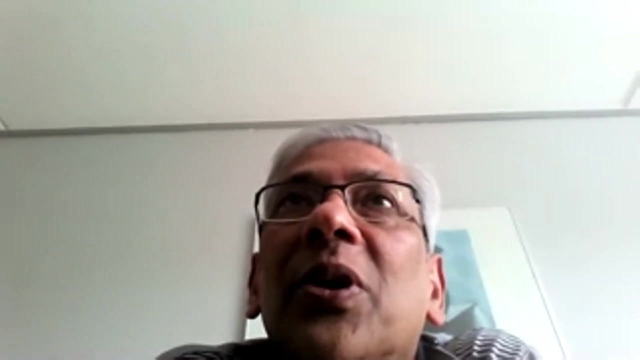 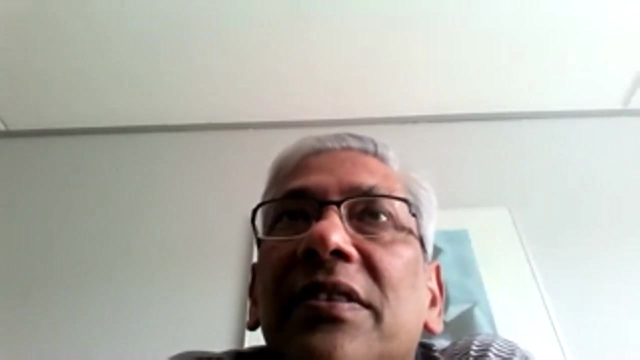 them into a consolidated conversion, stoichiometric reaction, pseudo reaction. And if we want any waste to go out of the system, we again can calculate the separation factor and identify it as waste. so it will go out vertically rather than horizontally, So it really doesn't matter at this stage. 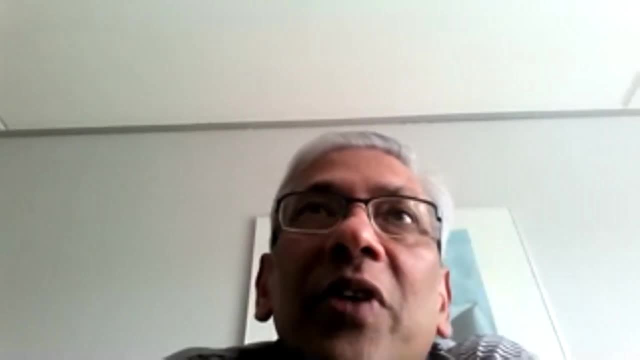 Okay, Okay, Yeah, But you could do this last question, Sure, So there is a separation factor that we use for the process. This is a process which is a to-to-to-to-to-to-to-to-to-to-to-to-to-to-to-to-to-the-to-to-to-to-to-to-to-to-to-to-to-to-to-to-to-to-to-to-to-to-to-to-to-to-to-to, the process. 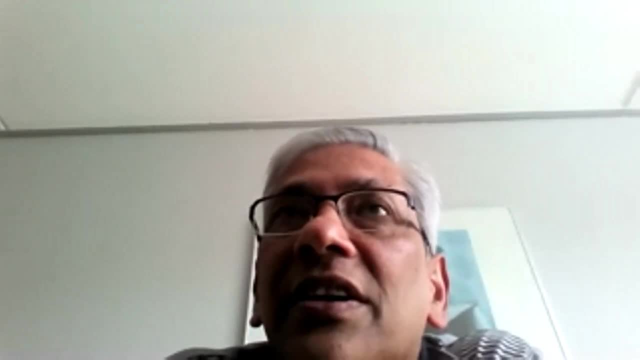 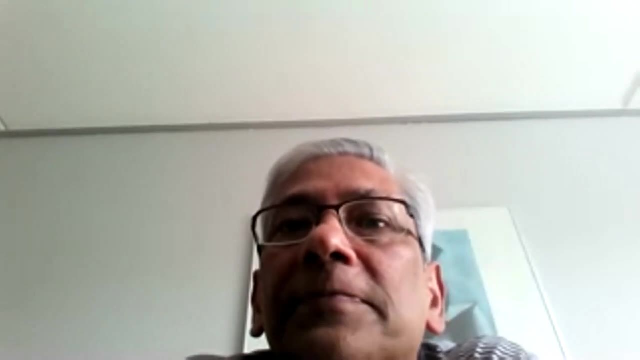 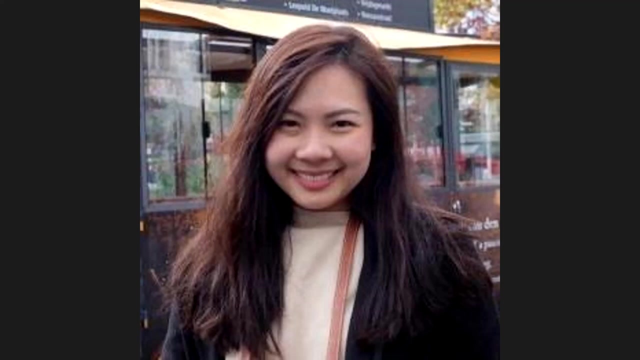 We could talk about the process group. It is one of our programs in JIMO, Which is the actual conventional unit operation, because in principle, with mixer, reactor, separator and divider, almost any process can be represented Is the process group also includes wind-based separations. 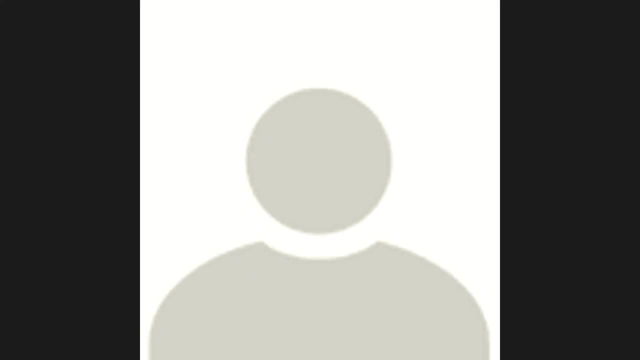 Sean, yes, We do have a process group related to liquid-liquid extraction and extractive distillation. right now we are kind of testing all those things and, yes, it will be soon be available for the users also. also, we do have a azotrope. 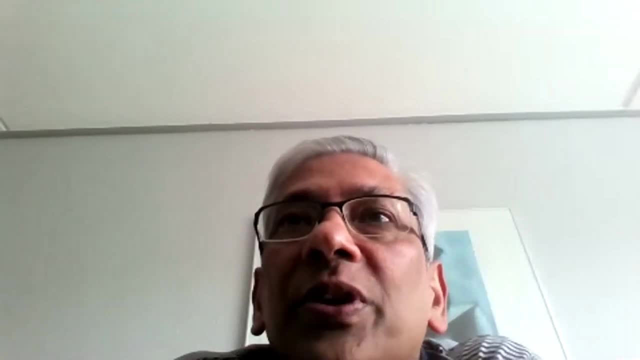 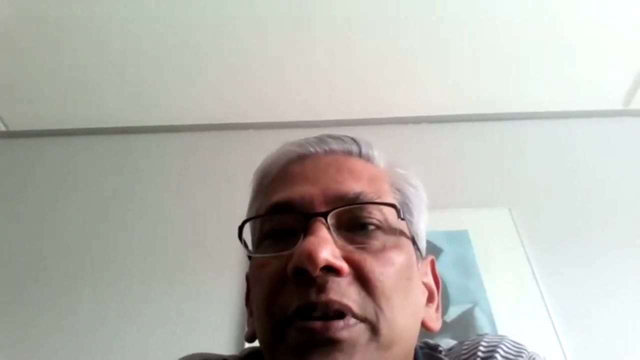 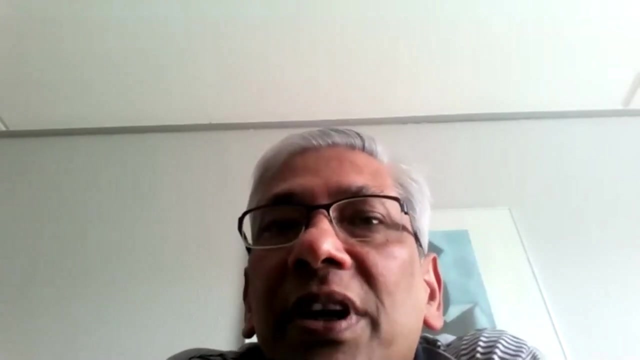 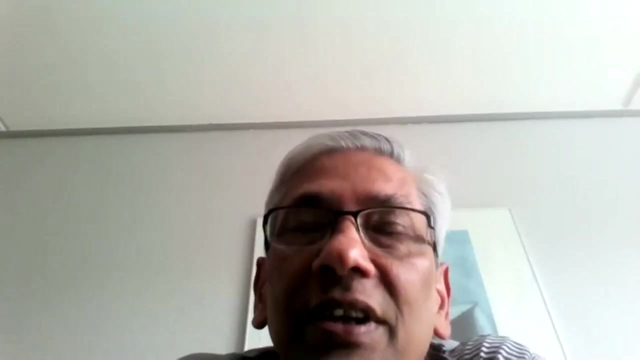 database or a program called azopro, so it will check if any binary pair forms an azotrope and then, based on the data, whether it is pressure sensitive or not. and for most of the homogeneous azotropes we have already found the best solvent and that is already in the azopro software. 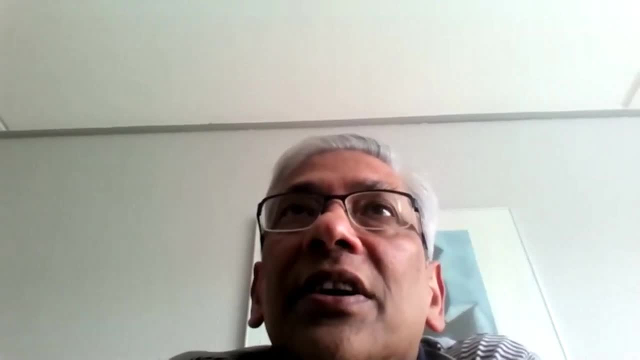 together with the process flow sheet for that. so the idea is that if we find azotrope and we want to use solvent based, we can just extract that part of the process flow sheet and add that to the workflow one that is generated in pro cft. 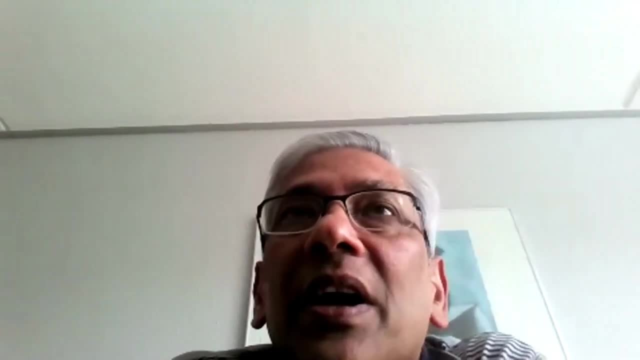 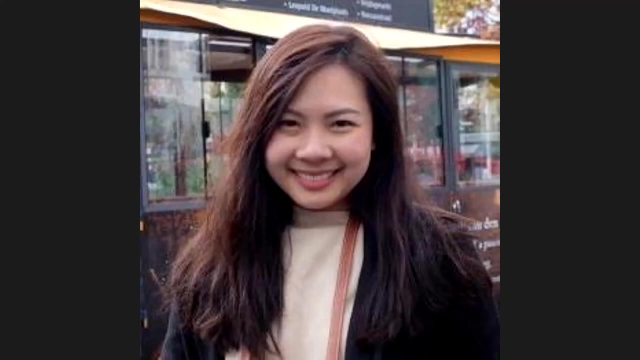 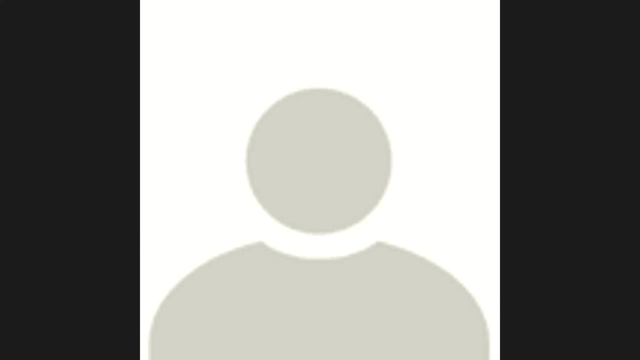 so at this moment, these are two separate tools, but they can be connected together. while developing this software, did you create your own chemical data or use some resources which are already available? i mean, while developing it, we have our own database and it has more than data for close to, i guess, 20 000 chemicals. um, so, yes, uh, these, these data were. 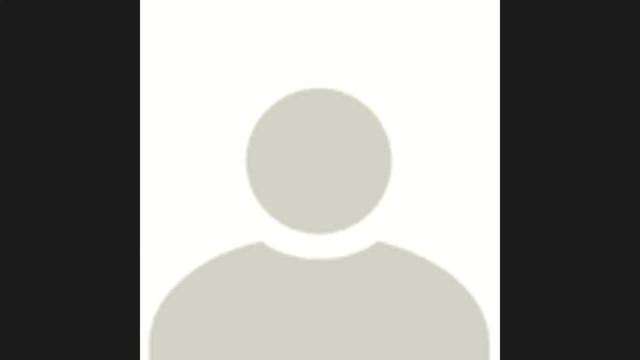 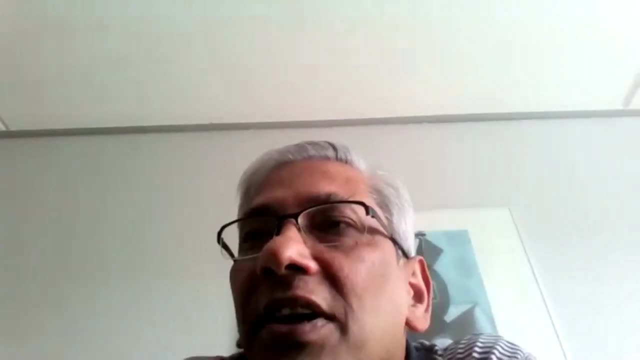 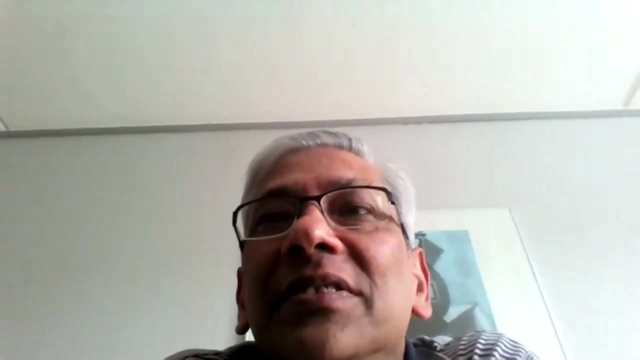 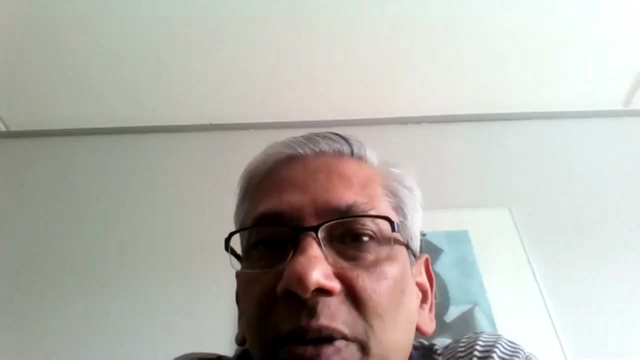 collected over the time of at least 10 to 15 years. yes, rafi, yes, yeah, so so we have our own database and i would say our database is more complete than others. maybe, but we are continuously increasing the database size because in the in the other webinars, like the product design, chemical substitution- 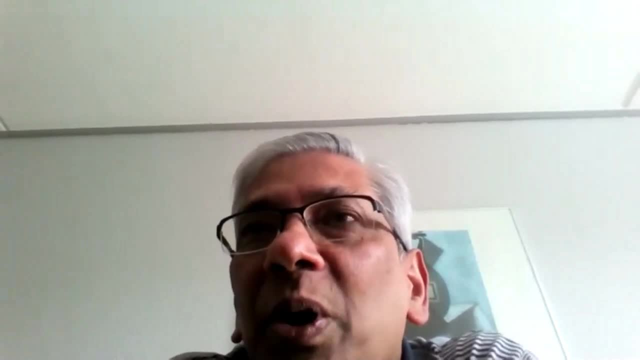 uh, there we need many more compounds and many more properties. so there is one database with uh 800 000 compounds but only 20 has data. the remaining 80 does not have any data except the molecular weight and the smiles. so we need need property prediction tools to fill them up. 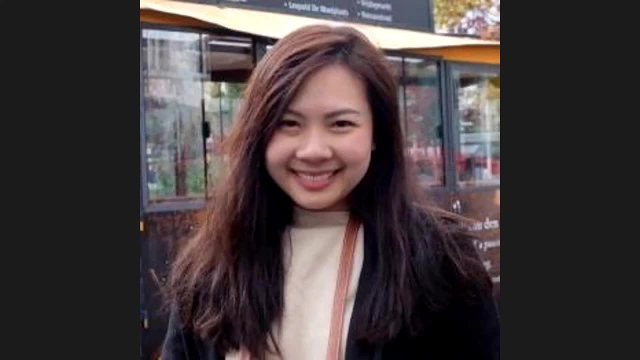 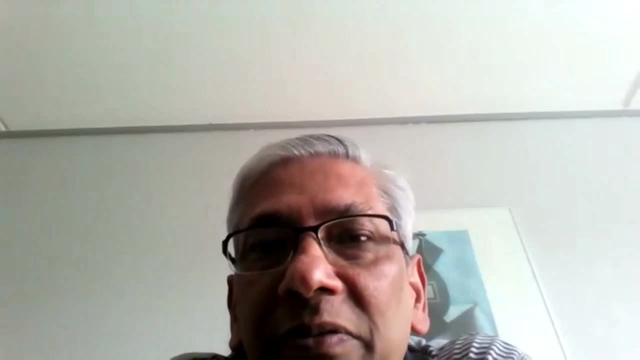 Are ionic separation being considered in software On this system at this moment? no, but we do have. you saw that in the background there was a ICAS simulator that was doing those. so we do have a reverse electrolyte system for which we 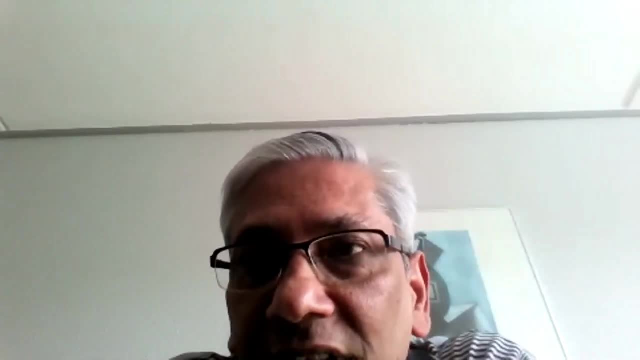 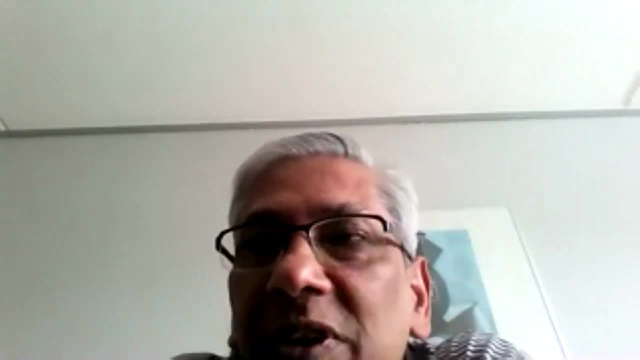 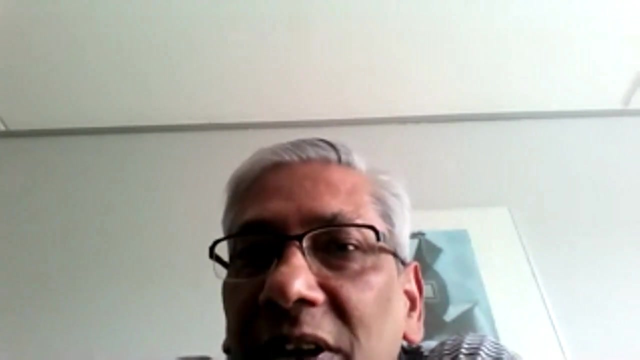 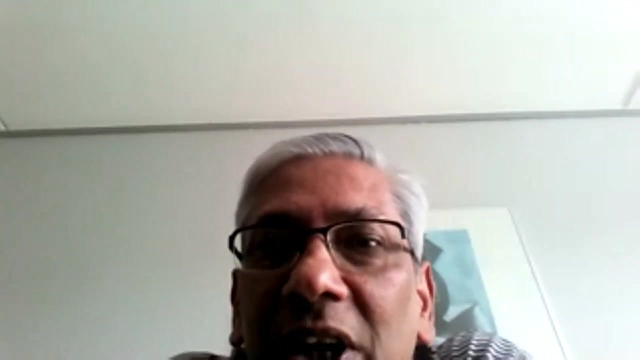 can generate the solid saturation diagrams and design the crystallizers. but we have not integrated that into ProCFD because we need to also design it so that it can be represented with mixer reactor, separator, divider, so that we can do it if somebody is interested. 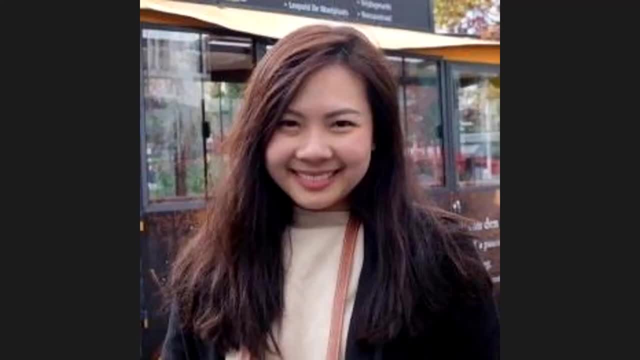 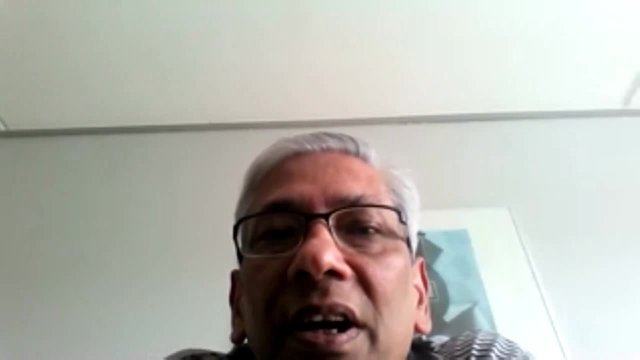 And last question: will the software only consider binary isotropes? No, actually it depends on how many compounds are there. If let's say there is four compounds and only one pair forms an isotrope, it's unlikely that there would be a ternary isotrope. 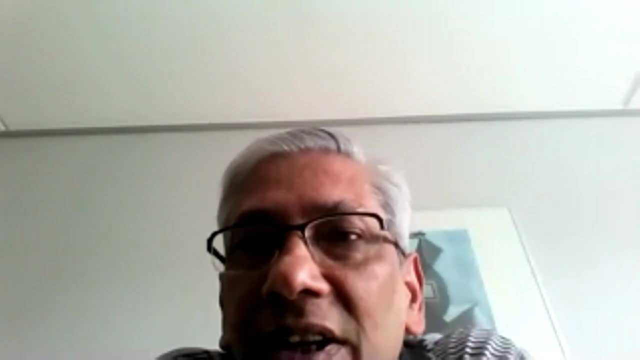 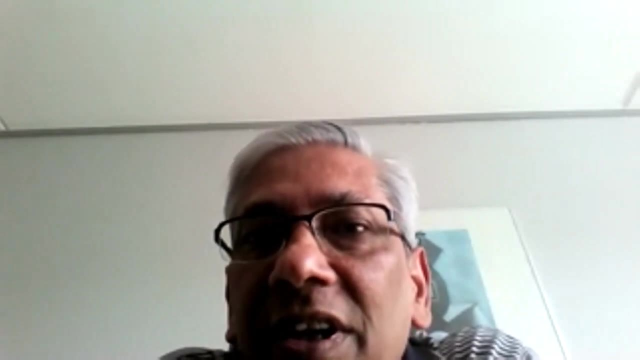 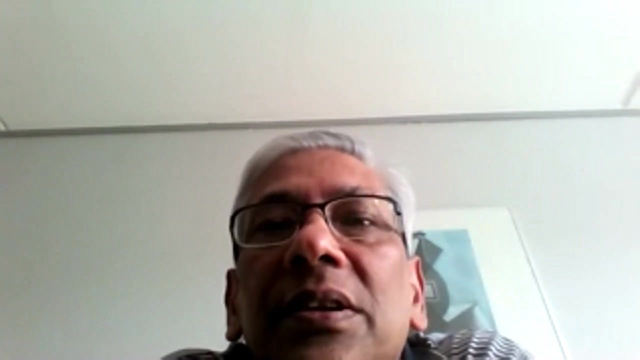 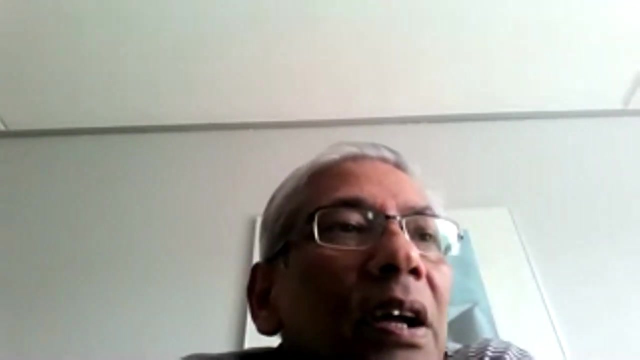 But if two pairs form an isotrope, then it could be that two binary pairs may form an isotrope. Then we have the means to check for the ternary isotrope. There are some more questions. Anybody has a question you can raise hand. 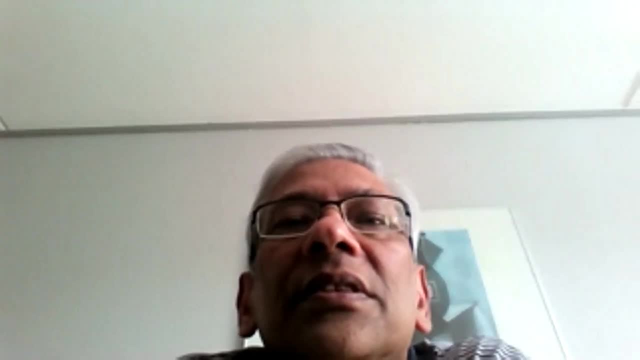 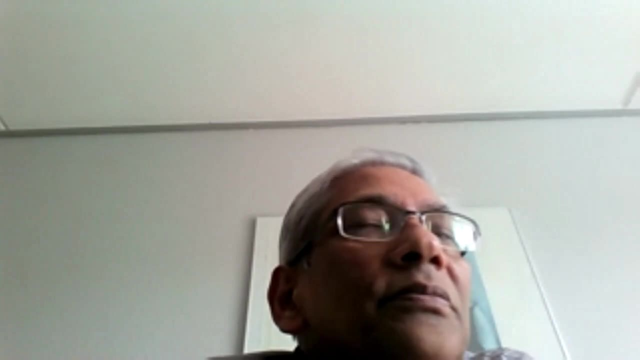 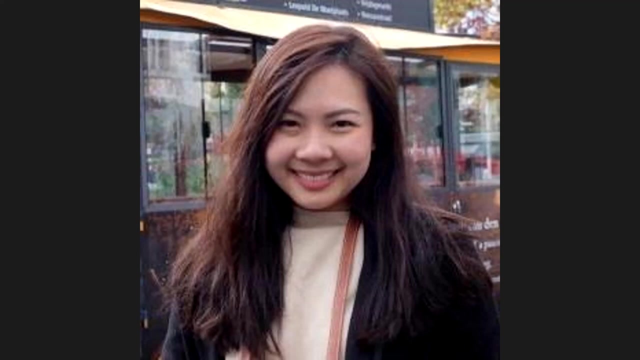 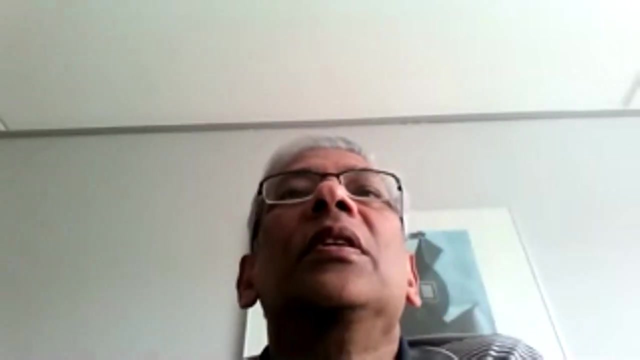 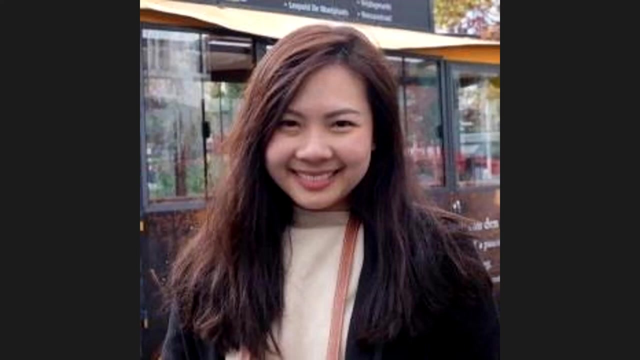 Okay, there is a question here says there was a raised hand somewhere. Participant 40,: Carlos, But there are some questions on the chat box, though, so from participant 58. Can you read it? Why does the preliminary economic evaluation did not become a parameter to add the ranking stage? 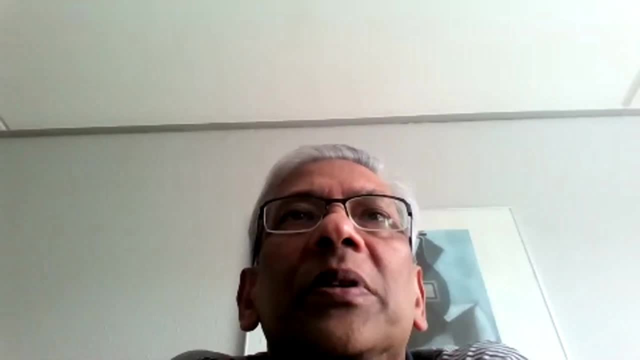 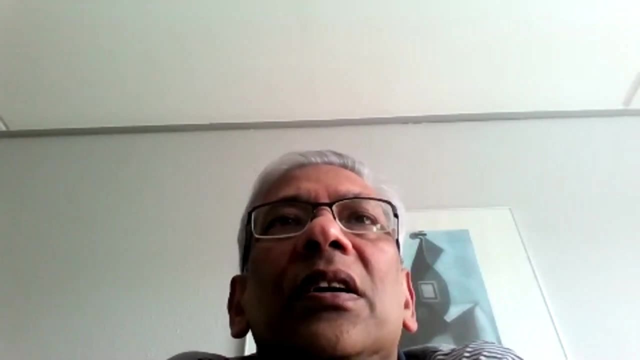 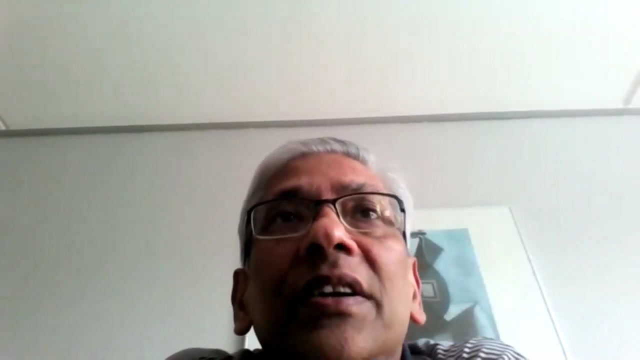 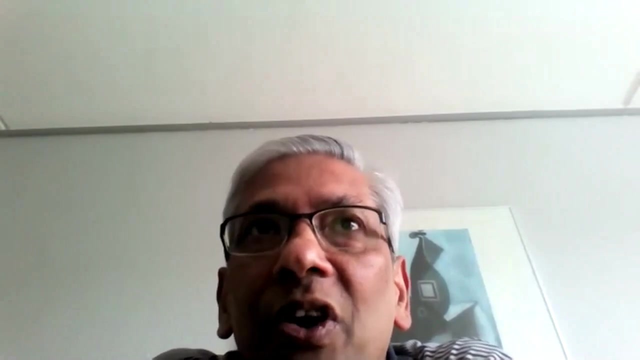 I'm not sure I understand the question. what is the preliminary economic evaluation At this moment? remember that, Yes, that's a good question, if I have understood correctly. Remember that we have not done any simulation at this moment because we have a flow sheet but we don't know if the separation 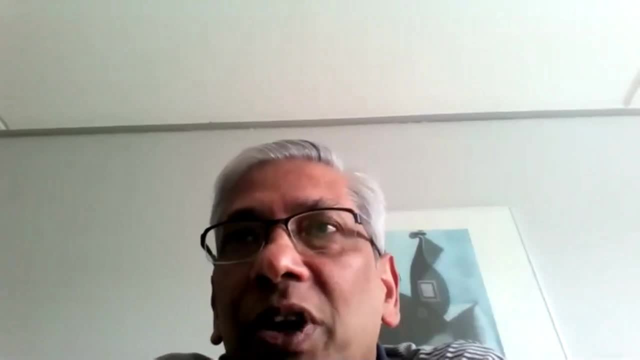 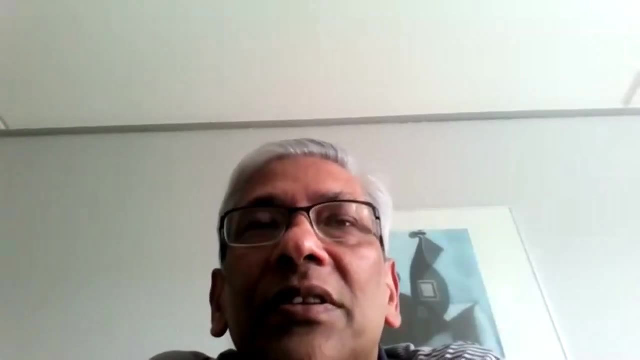 technique was distillation, what would be the number of stages, feed location and all of that? Before doing the simulation, we cannot do the economic evaluation, but we could actually, in the same way we generated the energy data, we might be able to generate the cost data. 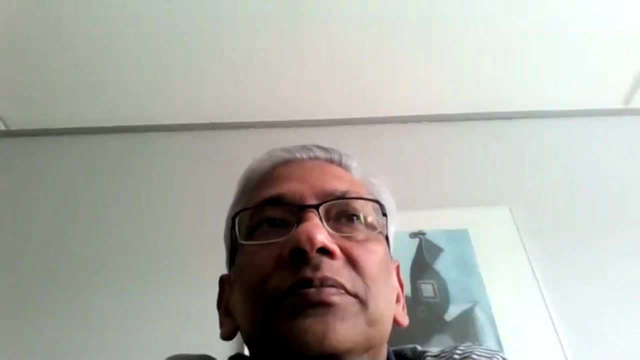 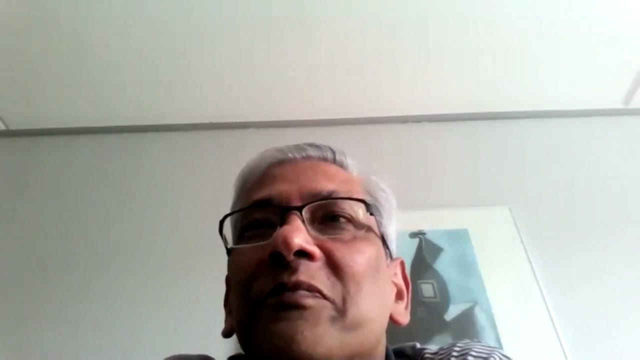 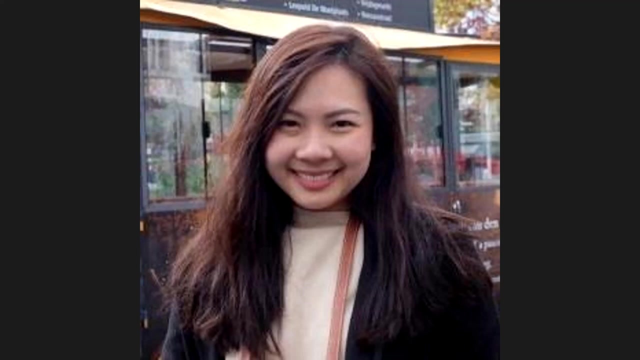 and make a good contribution method for the cost data. If somebody is looking for a project, I can give this as a project And you have a database of fatty acid, palm oil, biodiesel, graciline, etc. in your program, right? Yes, we do have a database of fatty acid, palm oil, biodiesel, graciline, etc. in your 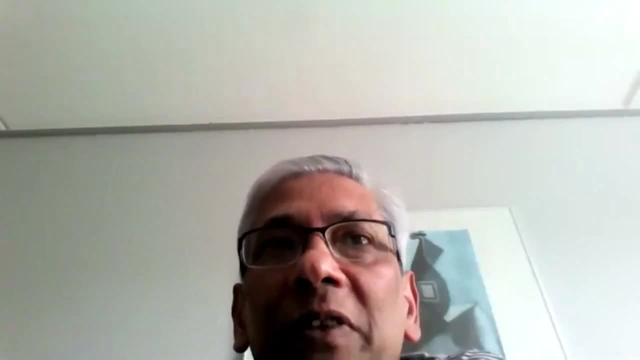 program right? Yes, we do have it. We have a special database. We call it the lipid database, and the lipid database, I think, is bigger and have better data than Aspen or Pro2.. But that lipid database will include fatty acids, palm oil, biodiesel, glycerin, all that, And we have connected. 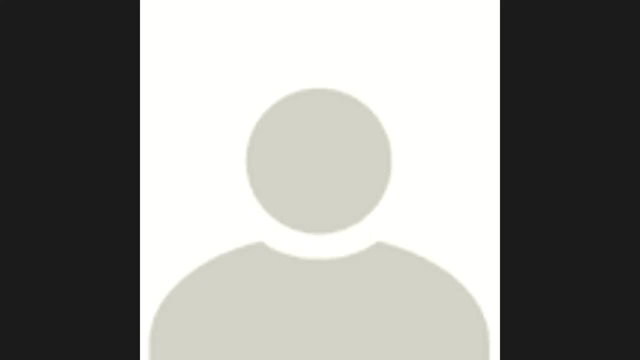 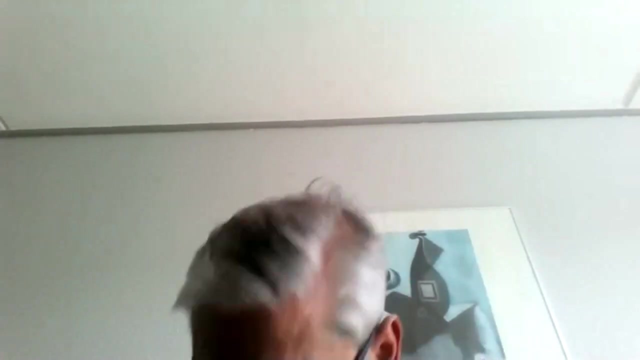 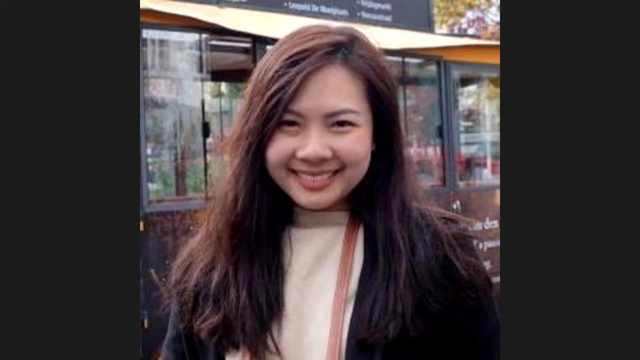 that also with Pro2.. Yeah, Not only properties. I think we also have estimation models and tools for that right For lipids. Yes, We still have time. So there are two more questions. Some people have asked me that the lecture and the recorded video will be posted somewhere. 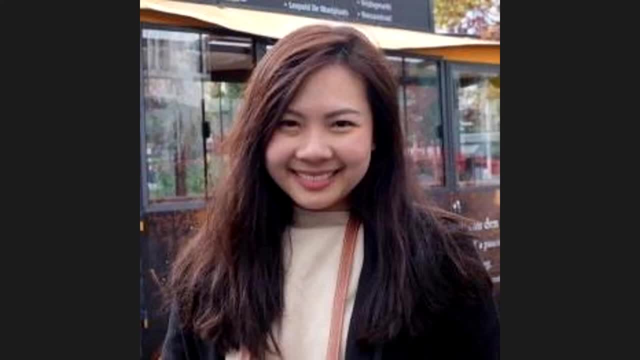 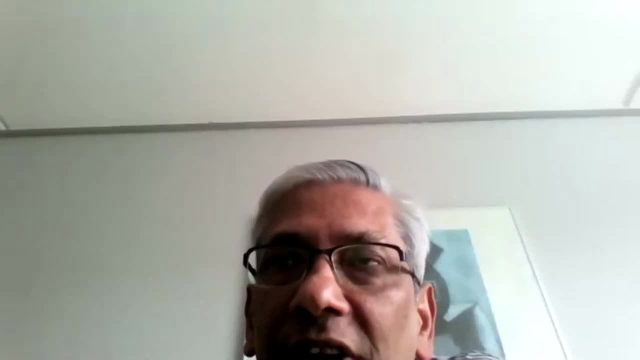 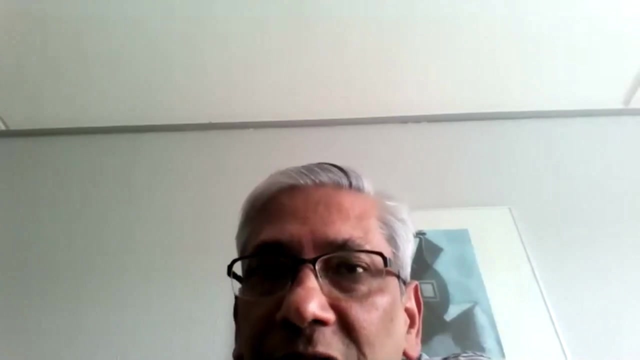 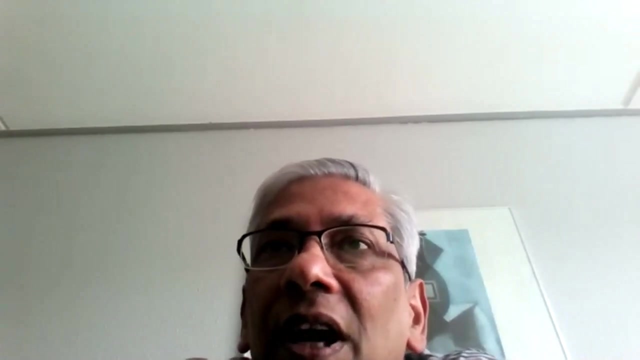 Yes, we will be posting on our website, right? Yes, So what we are trying to find is what is the best way to put those recorded videos, And we do have. PSE4Speed has a YouTube channel, And we would ask anybody who would like to. 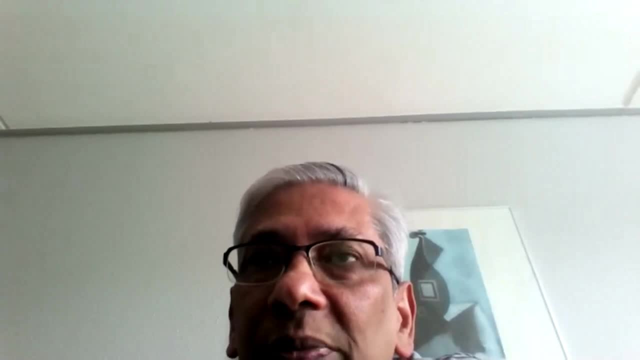 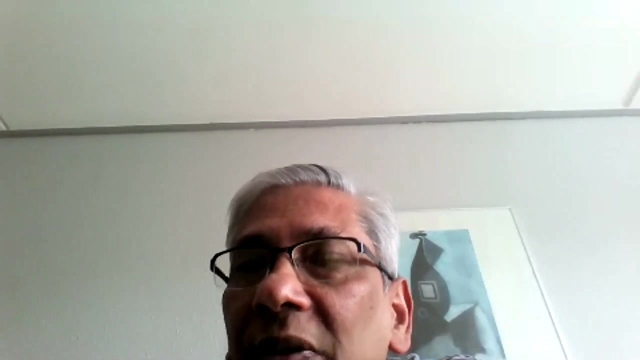 see those things? Yes, So what we are trying to do is to subscribe to our YouTube channel. It is free, But one has to subscribe, because that's how YouTube can see how many visitors we have, And then, once you subscribe, you would be able to access the recorded videos, And we have other videos. 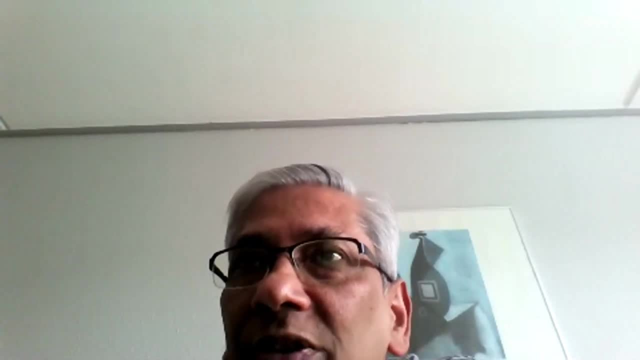 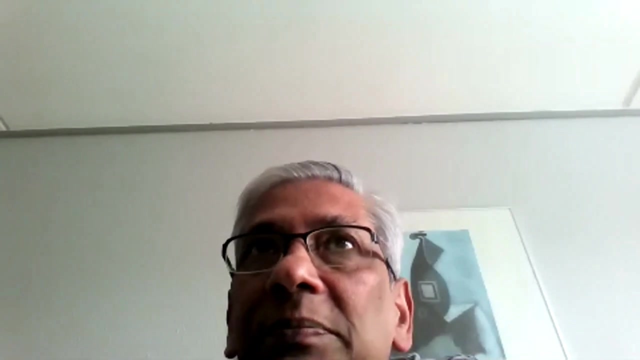 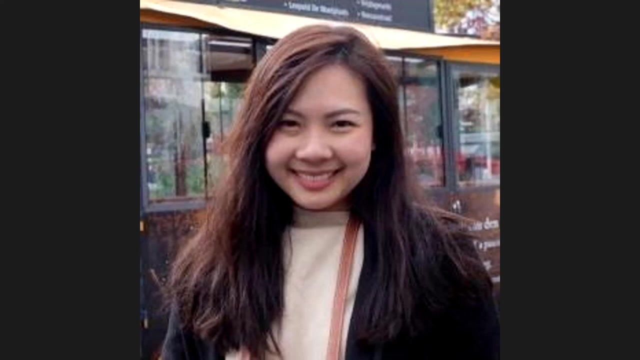 also that could be interesting for you. Yes, So we are trying to create this subscription-based YouTube channel. We already have the channel, but we are going to make it easier and better for any visitor to download them and use them. Another question is that, if you mentioned that you didn't use simulation method in this, 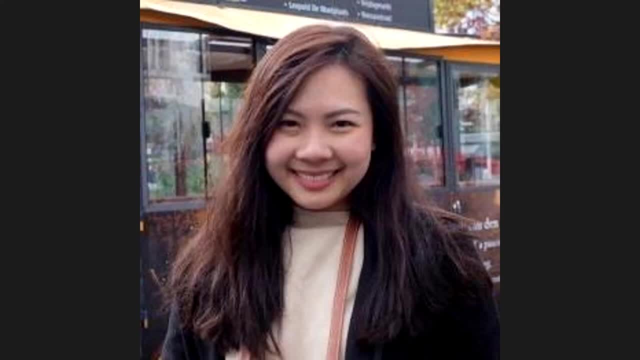 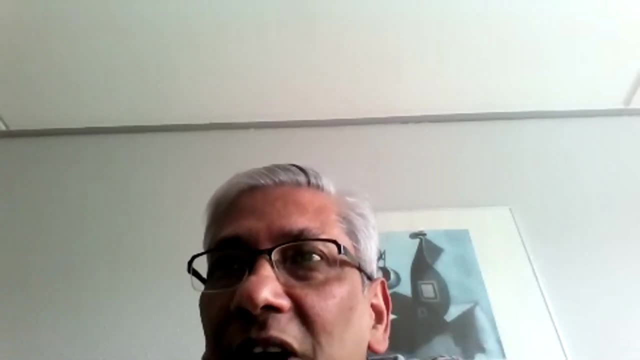 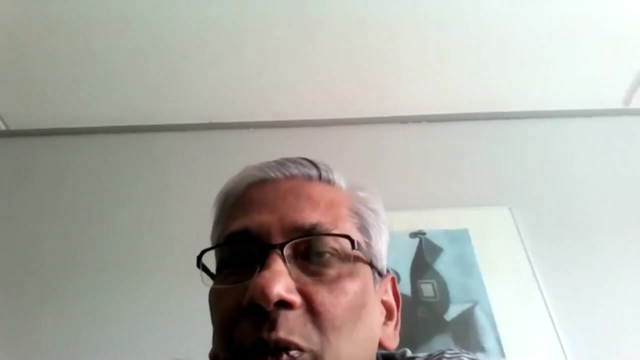 software Up to now. To now, Yes, Up to now. Tomorrow, you will see we will use simulation Because at this moment we are only ranking the process flowsheets And to generate the process flowsheets we have not used any data that would be needed for simulation And we have not generated any. 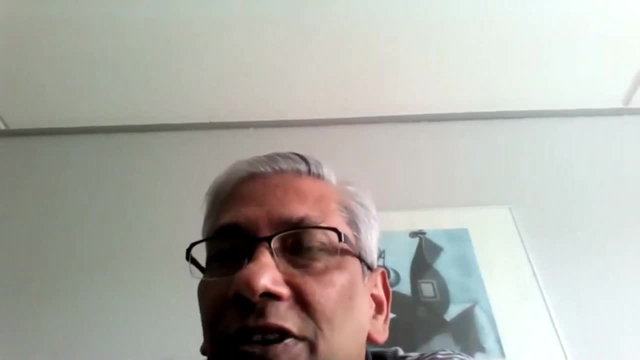 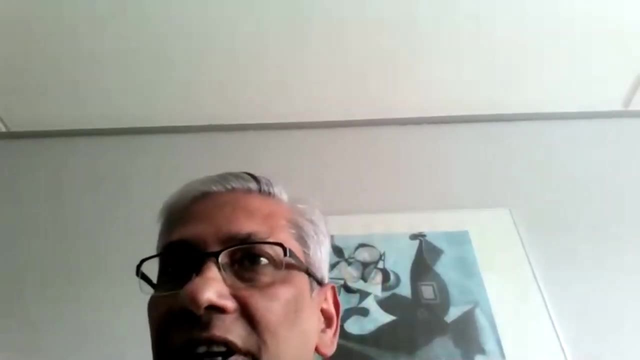 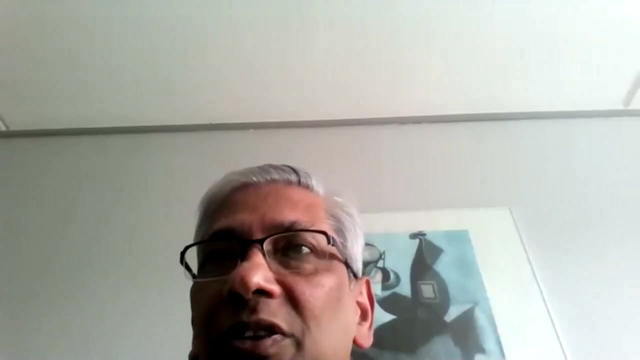 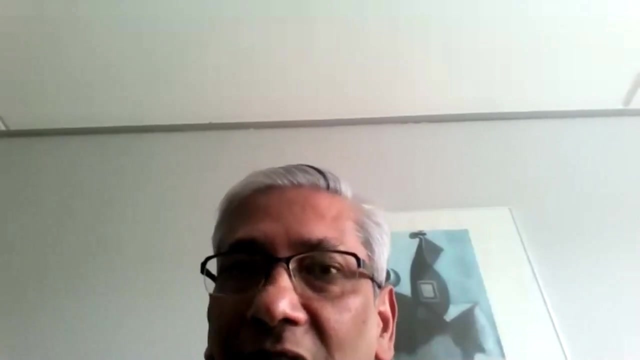 designs for the unit operations. So that's why our energy index and recovery, recovery and carbon footprint are based on group contribution method, in the same way that group contribution works for molecular property. But tomorrow the lectures will say, okay, if we have the 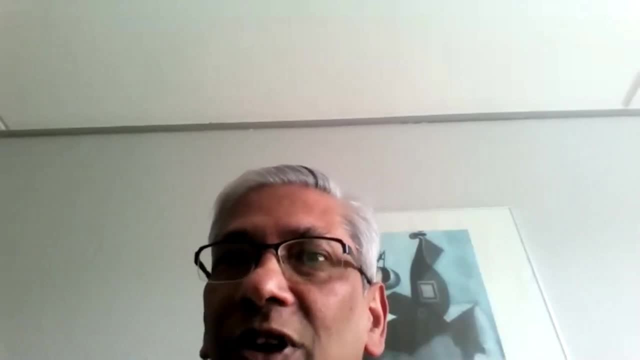 flowsheet. then for each unit operation in the flowsheet how to do the design, And then, once we have all the design parameters that are needed for a design, we will be able to go to the process flowsheet for a rigorous simulation of the process. Then we will actually 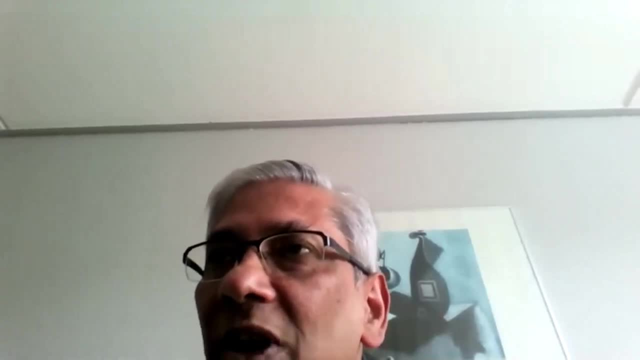 go to the process flowsheet simulator and simulate it. So the input file will be created automatically and the external simulator will be launched, And then, once the simulation is done, that simulation data will be then taken up by the cost calculation tool. Okay, 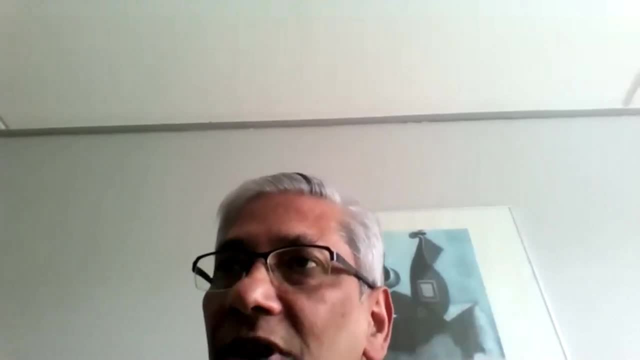 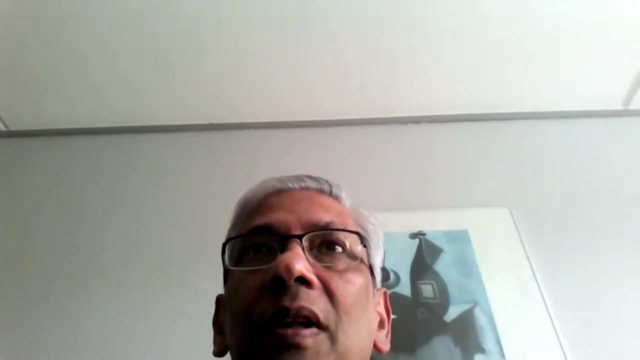 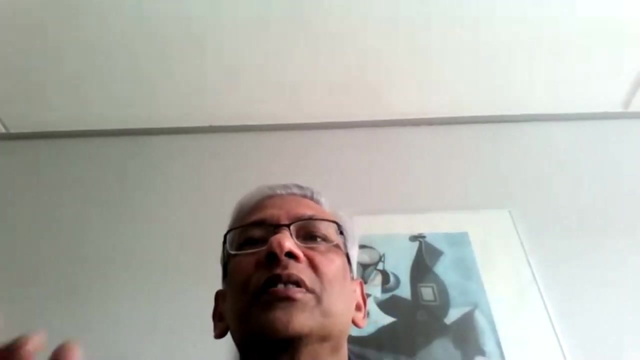 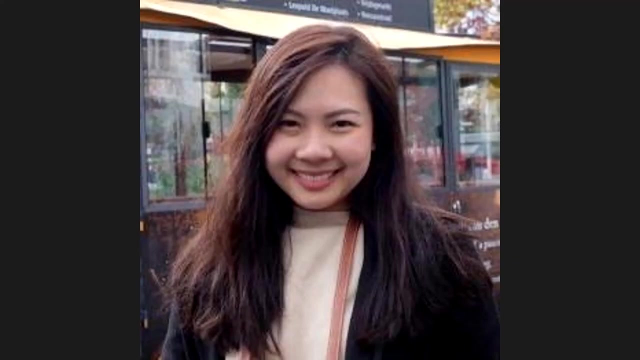 LC analysis to sustainability safety. all of these and then they all will be done. So all of these will be demonstrated tomorrow. Okay, Are there more? I see seven new messages. If anybody wants to ask the question with the microphone, feel free to just raise your. 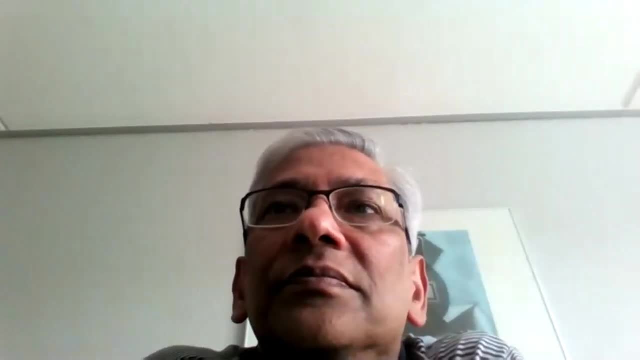 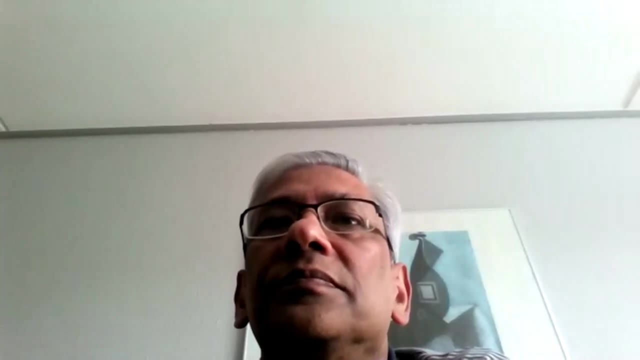 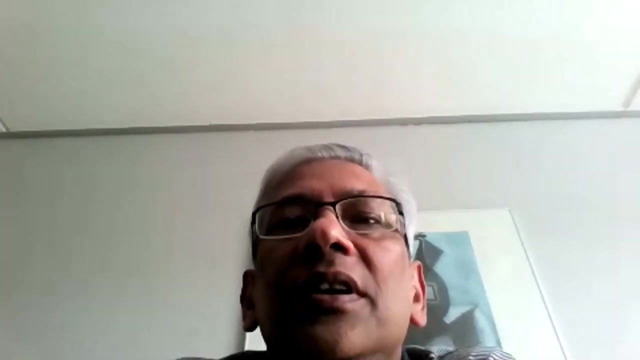 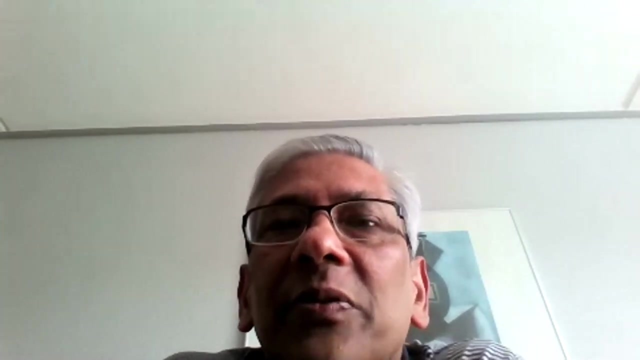 hand and ask your question. I can see one question: Can you share the link of your YouTube channel? Yes, I think it is in our website already, But yes, we will share it. Or, of course, maybe you can put as a message the YouTube channel link. 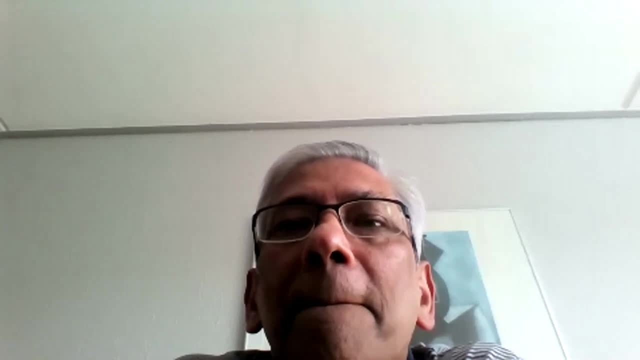 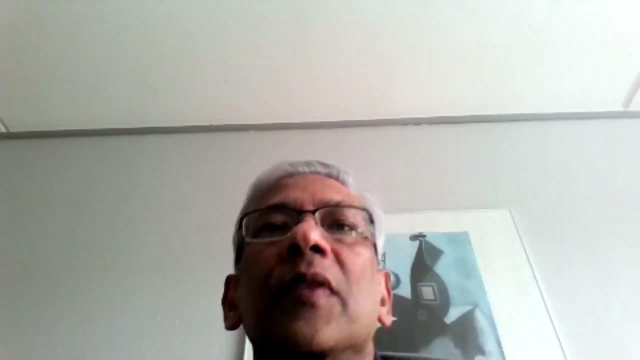 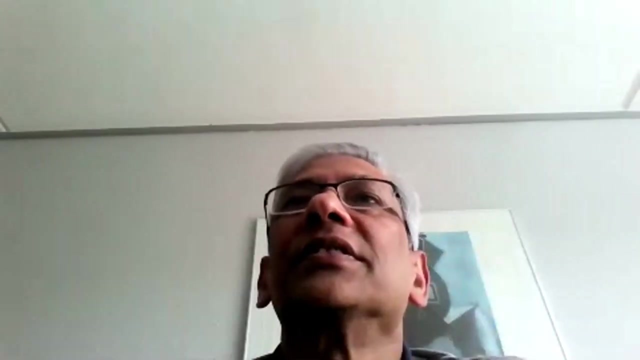 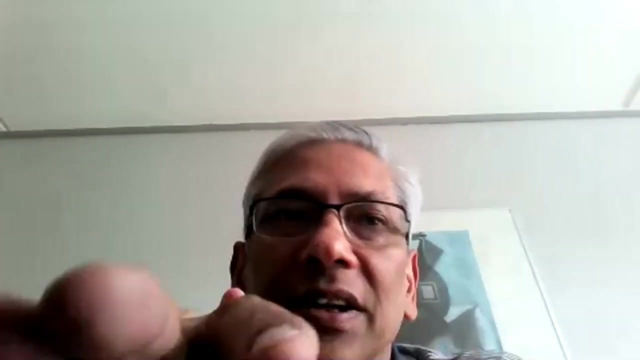 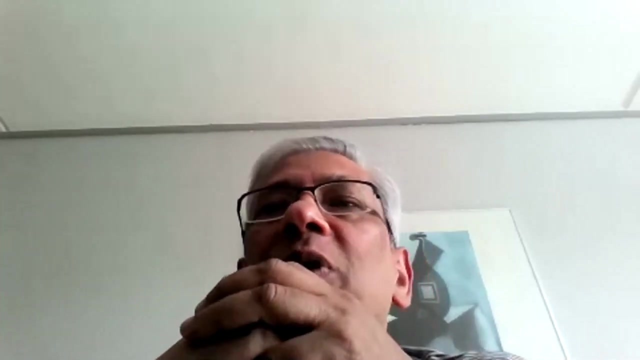 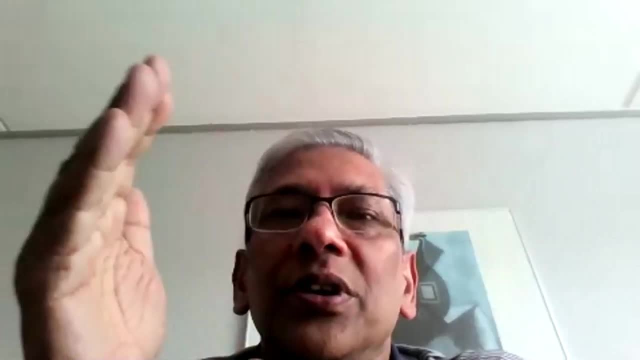 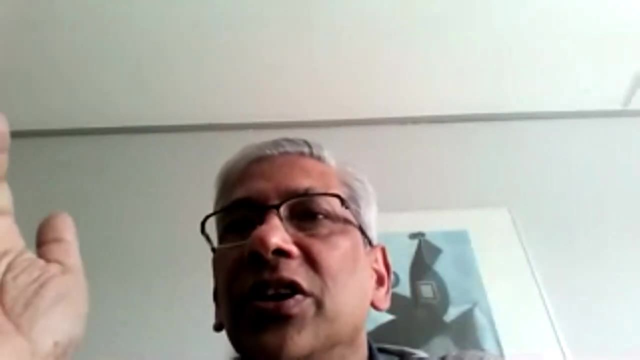 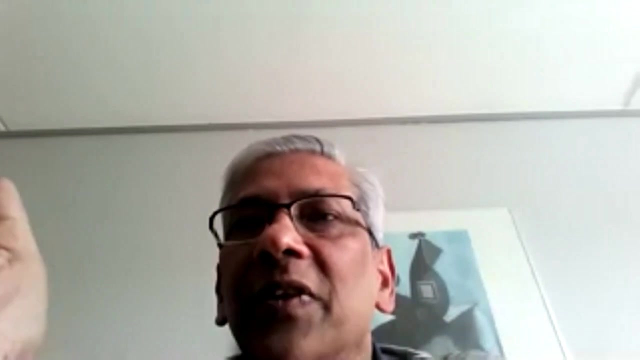 So tomorrow we will do from step five that you saw today: ranking of the flow sheet, all the way to analysis of the flow sheet, analysis of the process flow sheet, together with defining targets for improvement. So the idea is that we have a flow sheet, we analyze. 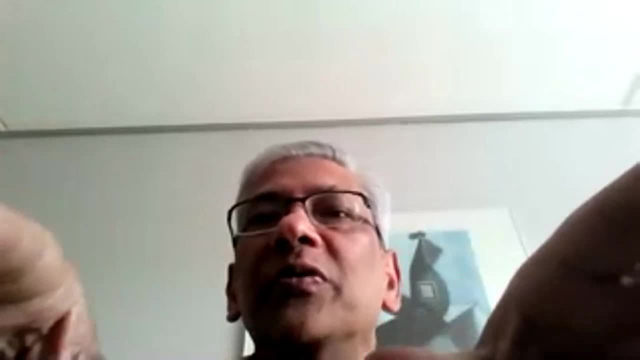 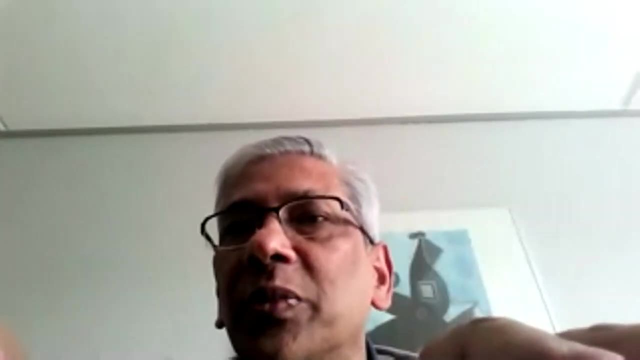 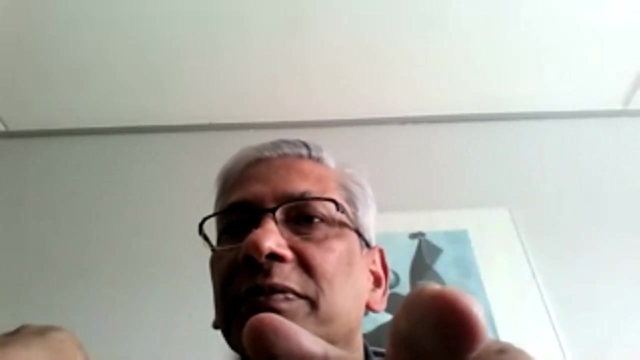 we find out how different ways we can analyze and improve the flow sheet And then we go to stage three, where we satisfy the targets for improvement And, by definition, if we satisfy the targets for improvement, it is a more sustainable alternative. So that will be in stage three.